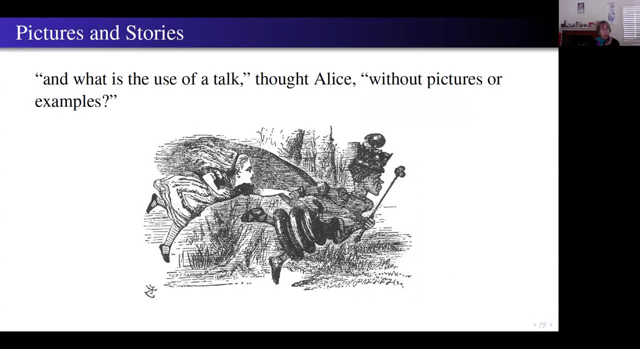 or conversations I usually translate into what's the use of a talk without pictures or examples. So today I'll mostly try to entertain you with some stories, And I hope that they're not only entertaining but perhaps also sometimes useful. Mostly these stories are about lessons. 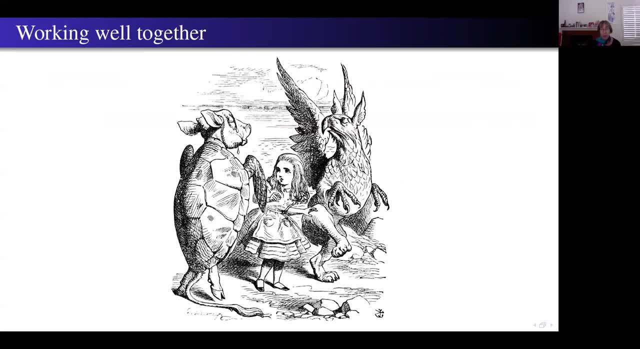 I've learned that I wish I had learned sooner, And one theme of this talk will be working well together. So the talk is entitled Mathematics and Cryptography- a Marriage of Convenience, And one of my collaborators said: well, maybe it's a menage a trois. since we've been talking about the importance of a marriage of convenience And I said, well, maybe it's a menage a trois, since we've been talking about the importance of a marriage of convenience And I said, well, maybe it's a menage a trois, since quantum. 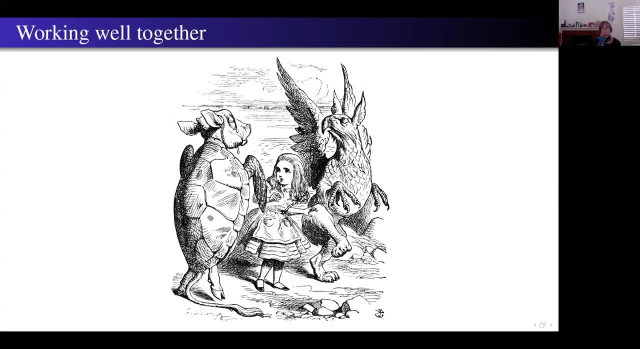 and post-quantum cryptography have brought physicists into the relationship, And another collaborator thought it really should be an open relationship, since it should include lawyers and politicians, And I think he liked the idea of an open relationship And there's a need for technical people and policymakers to learn how to communicate with each other. 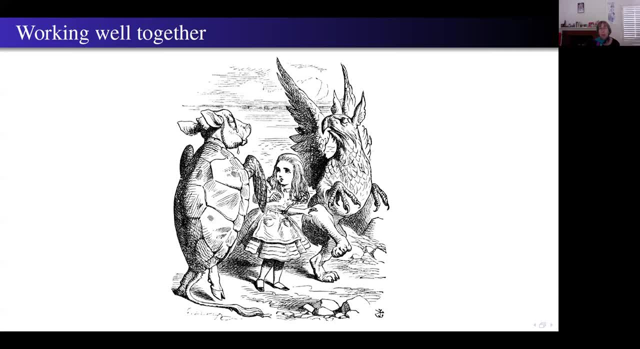 and build mutually beneficial relationships. So, as we're seeing, we're living in an interdependent world where everyone relies on everyone else, And we're more likely to survive and thrive if we can learn good ways to live and work together. So one good reason. 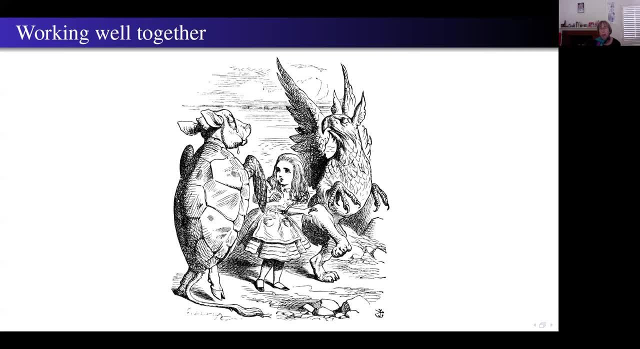 for mathematicians and cryptographers to learn to work well together is to make sure that we have good computer security and cryptography. So if a system's security is based on the presumed difficulty of some problem from number theory, it would be reassuring if the right 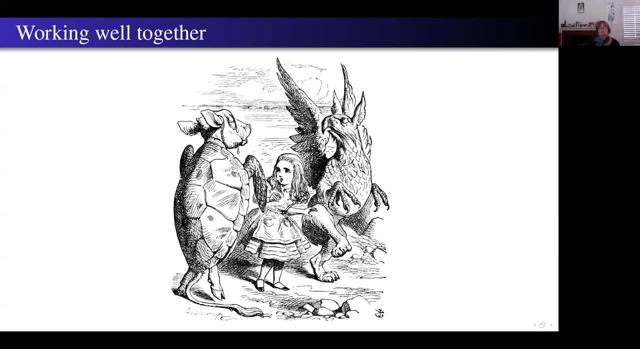 number theorists in the right field: first, know about the problem and second, try hard to solve it so that we have reason to believe that it might actually work. So I'm going to talk a little bit more about that in just a few minutes, and then I'll give you a little. 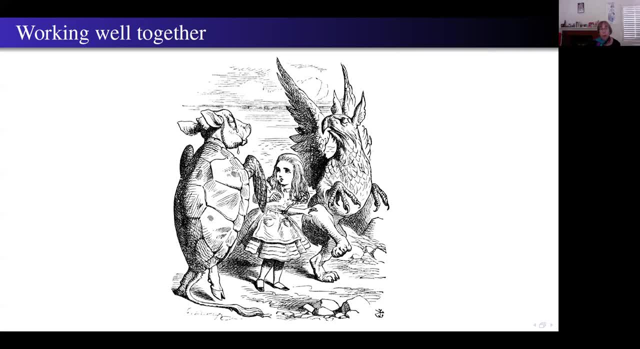 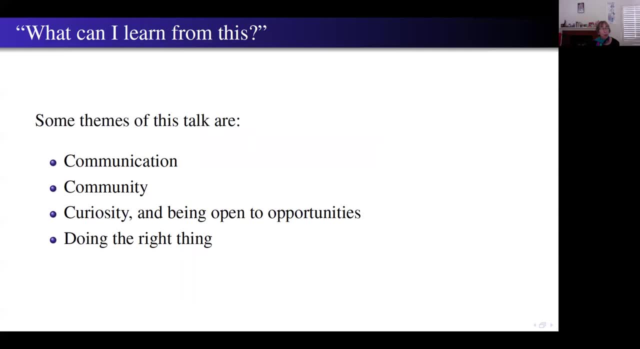 bit more detail on that. So for the sake of both good science and computer security, it's important to have good communication between the people who build our cryptography and the cryptanalysts and mathematicians who can test security. So for most things that I do or that happen to me, I try to ask myself: 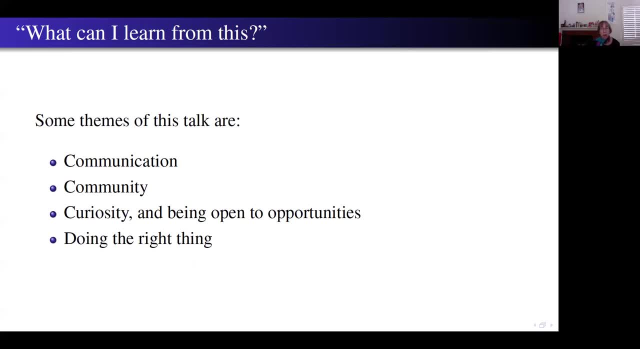 what can I learn from this? So if you want to ask yourself that about this talk, I'll just point out some of the recurring themes that you might notice. They're going to be communication, community curiosity and being open to opportunities and, of course, the 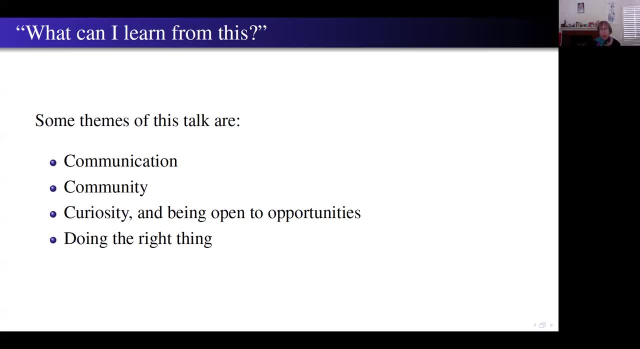 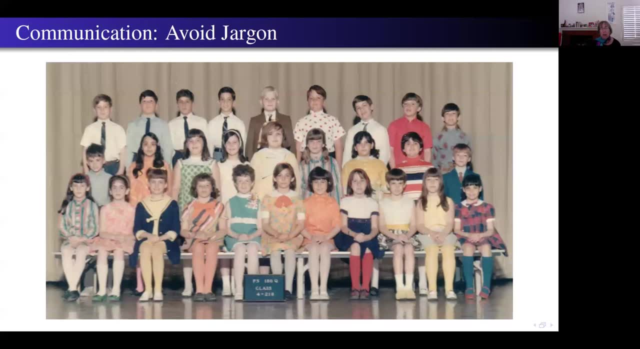 right thing. So I don't seem to have gotten very far down the alphabet, but maybe there'll be some later talk someday and I'll be able to do the rest of the alphabet, Okay. well, my parents didn't graduate from college, but they believed in the value of 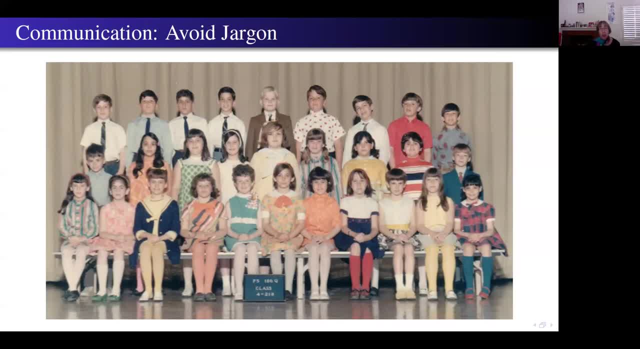 a good education. And I did manage to get a good education at New York City public schools, despite the fact that the city was on the verge of bankruptcy at the time. So this was fourth grade, But the story I'm going to tell you is I 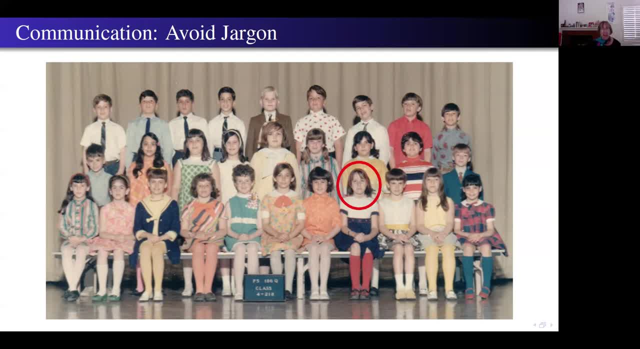 think from first year of high school. I was in the first year of high school and I was in second grade, but I didn't like the photo for that. So you get fourth grade. So I missed a few days of class and when I returned the teacher was talking about. 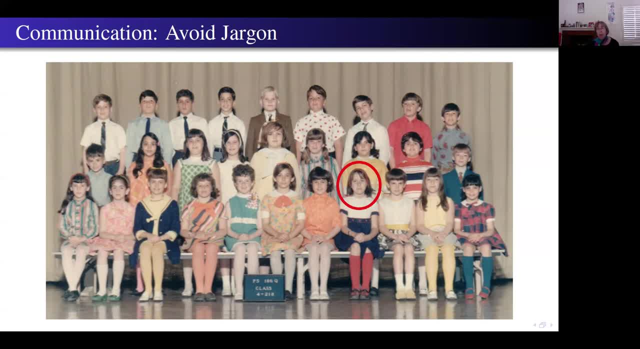 something called rational numbers And the students all knew what that was. but I'd never heard of rational numbers and I got really worried. didn't know how I was going to catch up and figure out what this was. So my friend Janet was sitting near me and I whispered. 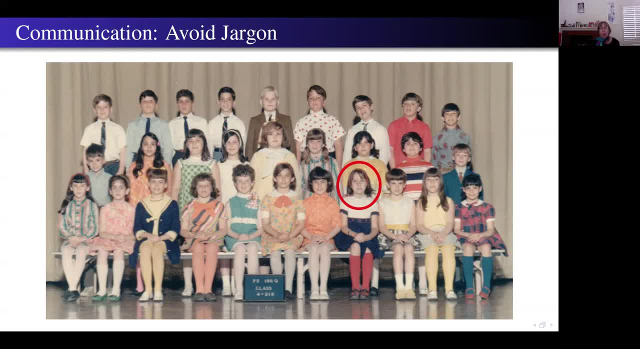 to her what are rational numbers? And she whispered back fractions. Well, this was clearly completely implausible. So fractions was a perfectly good word. Why would you come up with some new phrase to mean exactly the same thing? So this couldn't be. So she had to be wrong. I was sure I'd never find out what rational 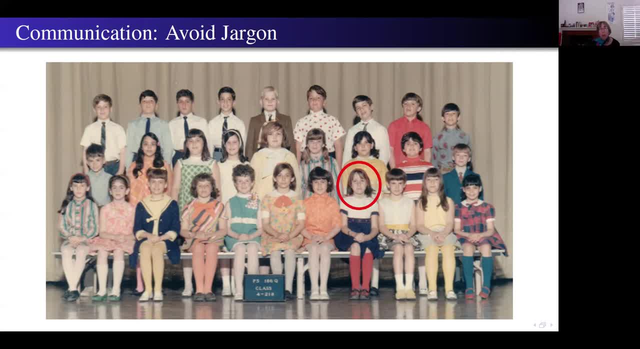 numbers were, I would fall hopelessly behind in math and never be able to recover. Well, that didn't happen, But since then I've been wary of unnecessary jargon. So I was on my high school's math team, which was an early experience that taught me the 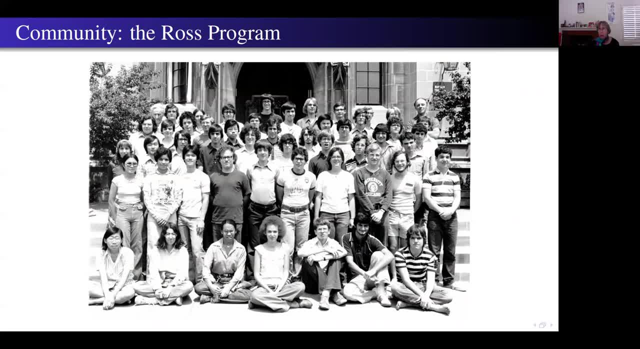 importance of community. And the other kids, including Stuart Haber, who some of you may know, told me about something called the Ross program. So that was a summer program for high school students And it taught exactly the elementary number three: that the cryptographers 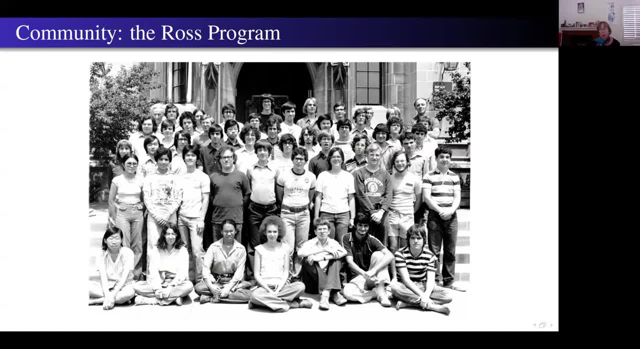 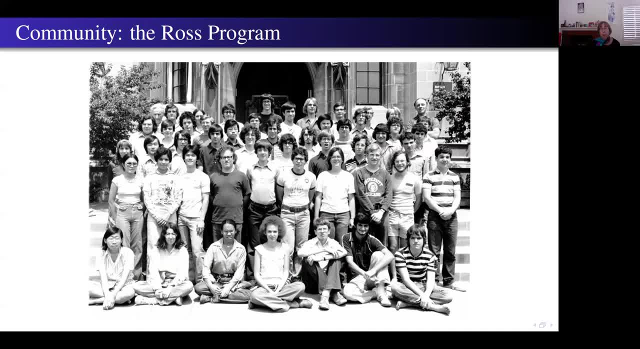 Even those that I met in that program. some of them have been helpful in my career and some are very important in my life. Some of the students went on to become mathematicians or computer scientists. Others became lawyers or doctors or went into other fields. Al Jean. 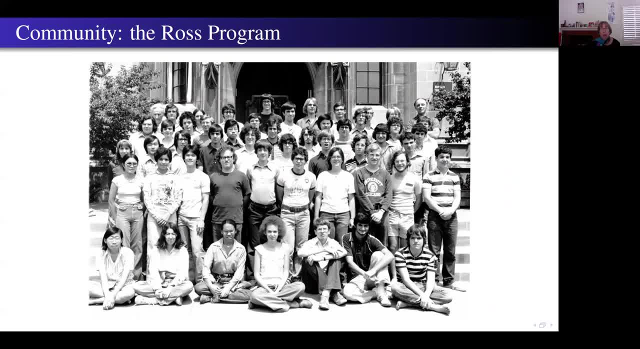 became one of the original writers for the television show The Simpsons, And in this program I learned the importance of correcting, clear proofs and good communication. And I went from being, as I went, from being a student to a counselor, to a seminar instructor. So as students, we prided ourselves in getting only four hours of sleep a night. 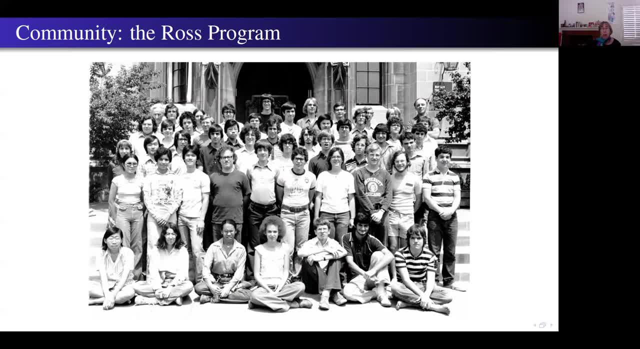 and working the rest of the time And later on. when I taught a problem session in the program one day, my students showed up and something was clearly different. And it turned out they had a test earlier that morning and had pulled an all-nighter the night before and hadn't gotten any sleep. So they were all 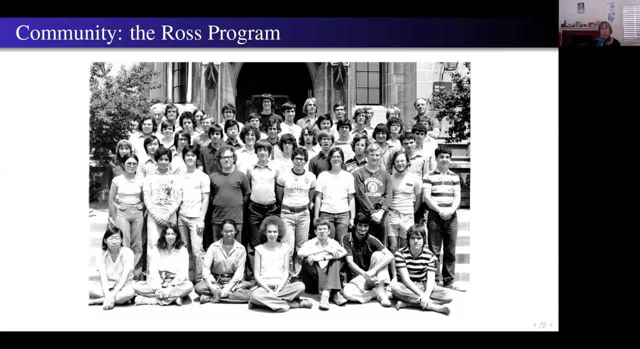 falling asleep in the seminar. So I asked them: which do you need most, a problem session or sleep? And they all said sleep. So I turned out the lights and that made it pitch black because there were no windows. They put their heads. 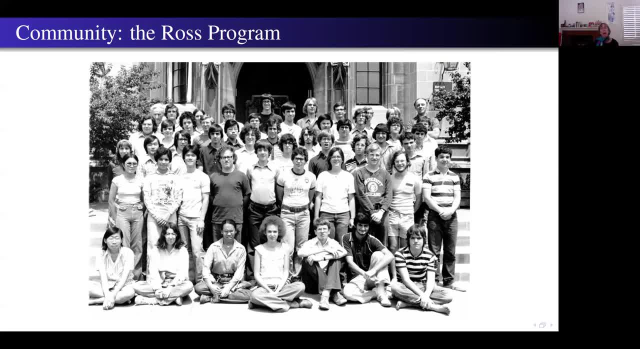 down on the table. some of them even lay down on the floor and they went to sleep And that was what they really needed. So I'm glad I listened to what the students told me. Sometimes you just have to stop everything and take care of your health. 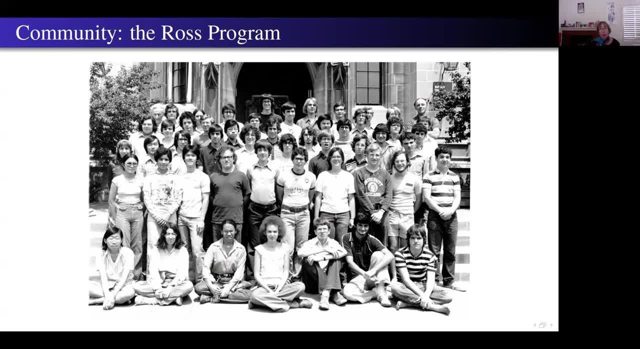 And the best advice I can give students and more generally everyone, is: your highest priority is your health. get plenty of sleep. And then I asked them: what do you need? And the answer is you need to work and eat well and maybe listen to other people find out their needs. 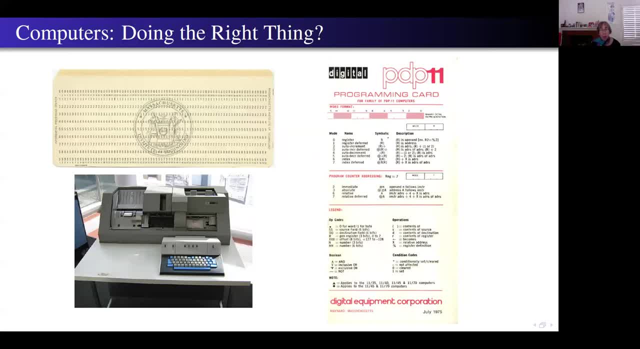 Well, my undergraduate college did not have a computer science department. at that time There was a high-powered programming course in the applied math department. but since I didn't have any background, I decided I better first cross register for a course at MIT. and there I learned. 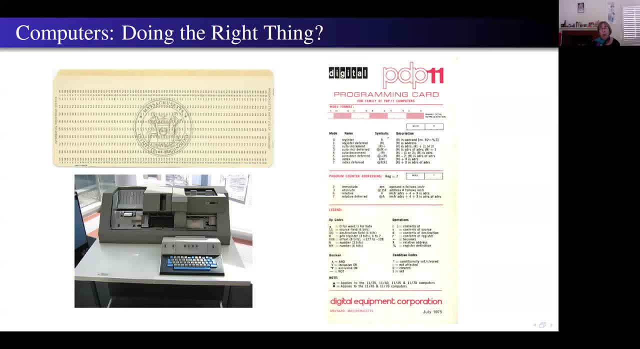 Fortran using punch cards. So then I took the high-powered course where, among other things, I learned to program the PDP-8 and PDP-11 in machine language and assembly language, which has been completely useless for me and I don't remember any of it. But what I do remember is that we had 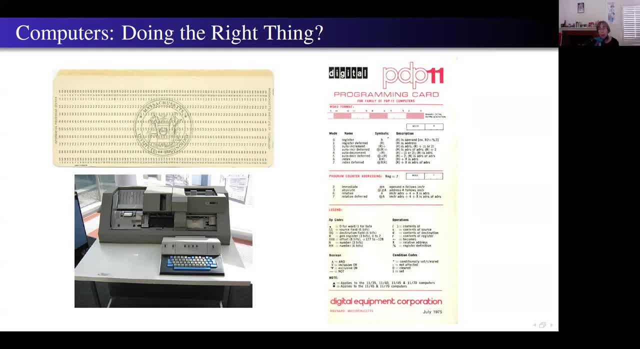 really annoying quizzes, where the idea was to write down a short program in 10 minutes, but we were allowed some what seemed to me ridiculously large number of mistakes. I don't remember if it was three or five. Now I could write down a completely. 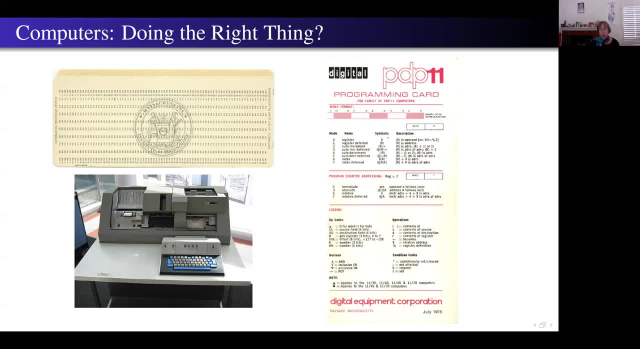 correct program in 12 minutes, which meant 10 minutes to think and plan and two minutes to write it down. So I thought it was terribly unfair that there was no reward for taking that extra two minutes to get it right. So after 10 minutes I hadn't written anything. 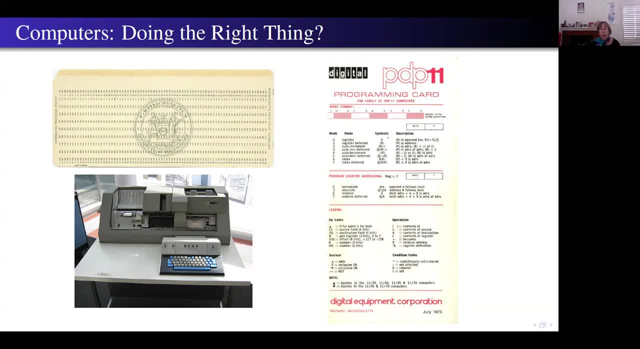 and the test was over. So you know, for our homework assignments, the other students would spend maybe half an hour writing the program and maybe 16 hours debugging it. Well, I can write it in, you know, twice the time in an hour, but I didn't know how to do it. I didn't know how to do it. 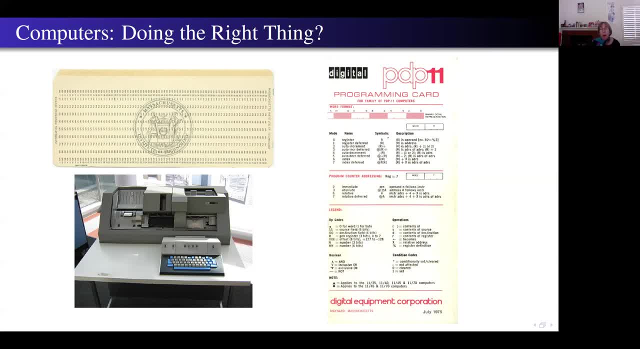 I spent considerably less time debugging, So I'm reminded of this idea that fast and dirty is better than slow and careful. when I think of publishing and competitive conference proceedings versus publishing in journals, So I think of it as the tortoise and the hare, So I think better. 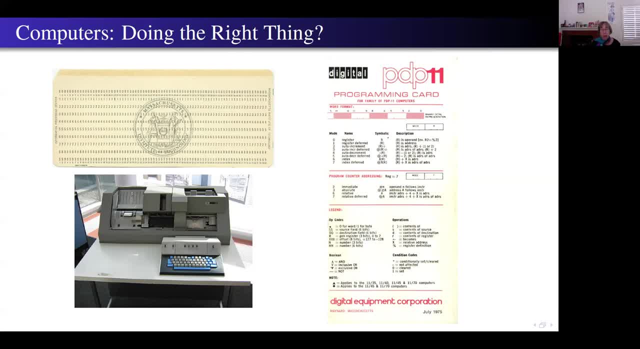 work gets done when there's time for referees to fully check the work and for some back and forth between the referees and the authors to make sure papers are correct and well written. So you know the output might be better than research, and under tight deadlines with page limits and short time frames for reviewing. 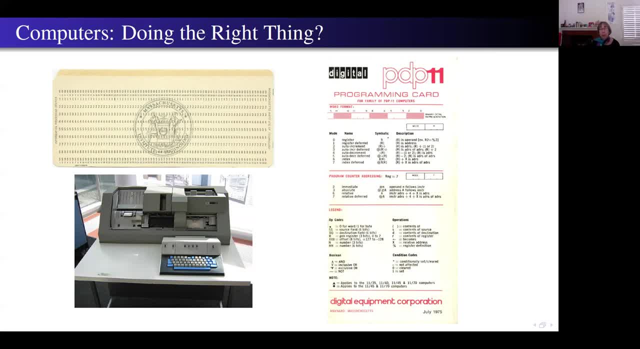 And I'm also a great believer in using experts, sending preprints to the experts, putting preprints online and getting feedback before publishing. So it might make sense to cut down on the number of conferences, especially given we might not be able to go to conferences. 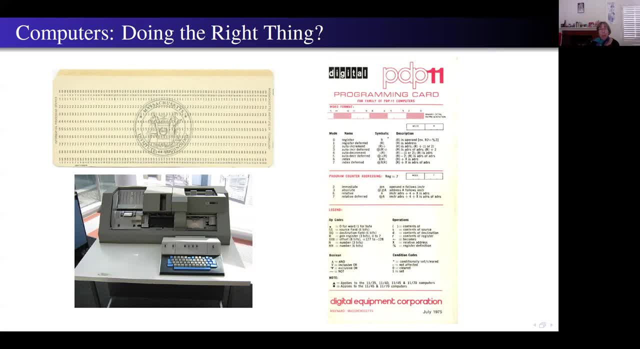 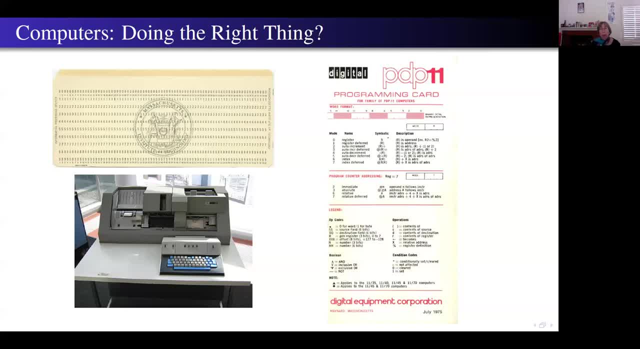 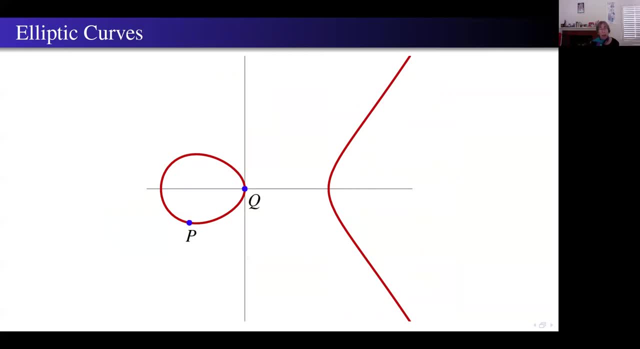 are appropriately rewarded for reviewing. that's both good and timely. Okay, I went on to do number theory, in particular elliptic curves and abelian varieties, which are the higher dimensional generalizations of elliptic curves. You don't need to know what they are for this talk. 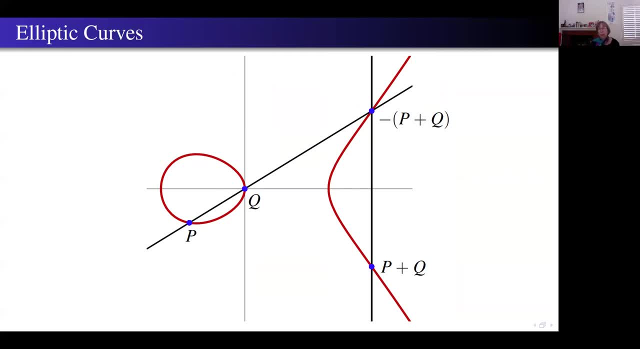 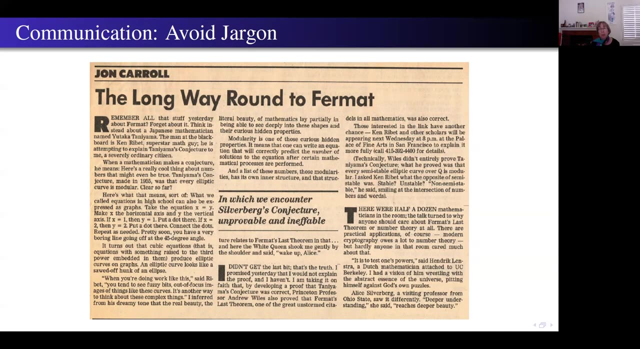 I'll just say that elliptic curves are useful for cryptography because they're defined by a simple polynomial equation, So they're easy for a computer to handle and they have a useful addition to them. Okay, so I went on, did number theory When a proof of Fermat's Last Theorem was first. 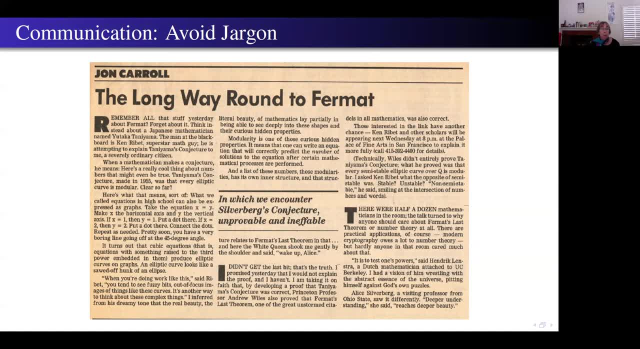 announced by Andrew Wiles, a reporter for the San Francisco Chronicle, came to the Mathematical Sciences Research Institute in Berkeley and interviewed a group of us. Now one of the mathematicians explained Fermat's Last Theorem by saying that certain equations have no non-trivial. 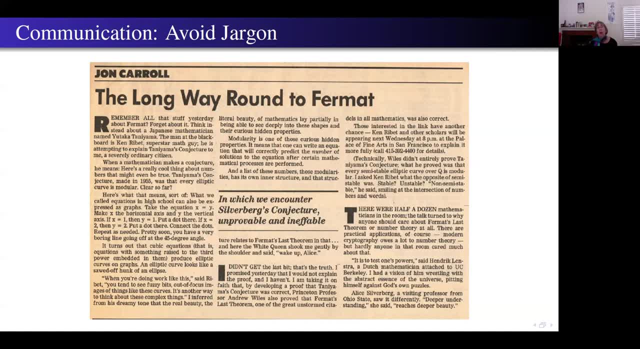 solutions that are rational numbers. And he kept using the phrase rational numbers. So I looked over at the journalist and saw that his eyes had glazed over and he'd stopped listening. So I leaned over and whispered. when he says rational numbers, he means fractions. 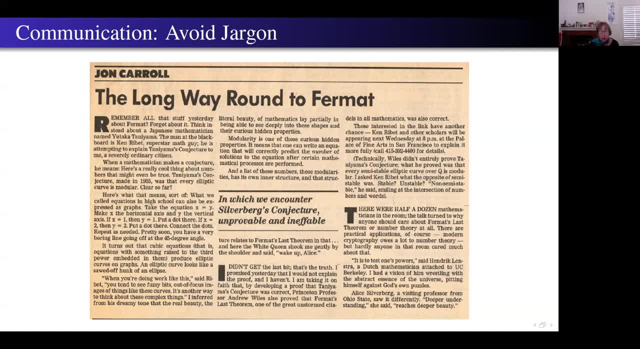 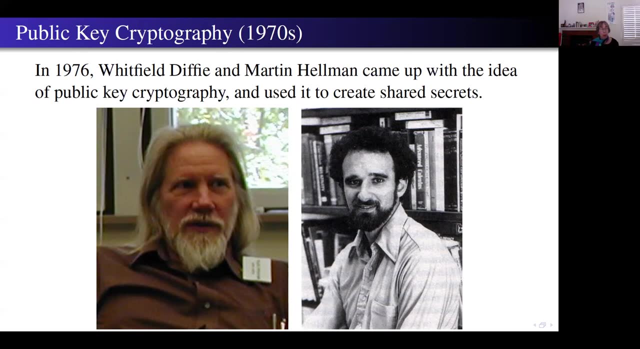 And the reporter breathed a sigh of relief and said thank you. So again, it's important to keep in mind that people from other communities might have a different vocabulary. Well, as most of this is known, in the mid-1970s, Whit Diffie and Marty Hellman came up with the idea of public key. 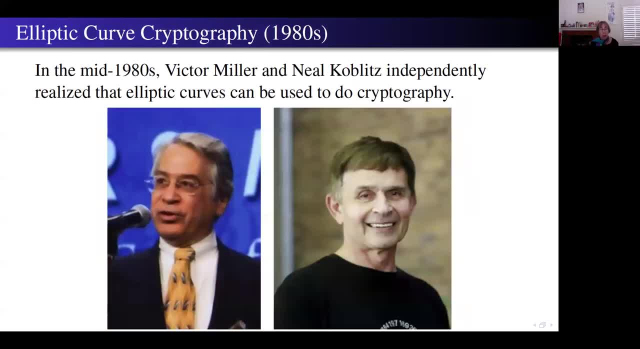 cryptography and used it to create shared secrets. And in the mid-1980s, Victor Miller and Neil Koblitz independently realized that elliptic curves can be used to do cryptography. They can be used to do things like Diffie-Hellman key agreement, which I'll talk a little more about later. 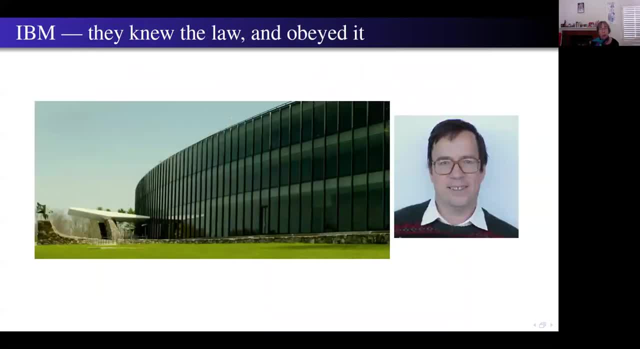 So soon after that I had the opportunity to spend a year at IBM, So that was in the late 1980s, And the people I interacted with the most there were Victor Miller, who you saw in the last slide- he was my mentor that year- and Don Coppersmith, seen here, And my first cryptography talk was 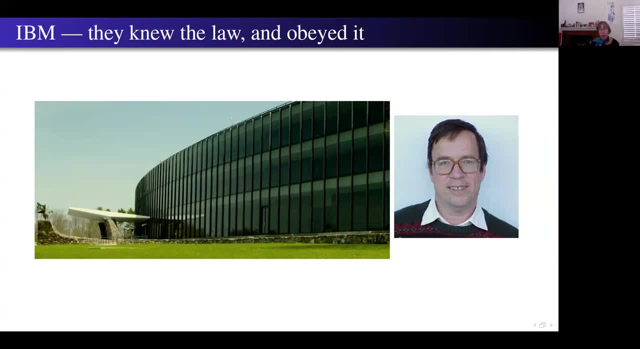 actually a survey talk I gave at IBM on elliptic curve cryptography with Victor Miller in the audience, which I'm really embarrassed to think about now, since he was the expert and certainly knew a whole lot more than I did. So why do I call this slide? They Knew the Law and Obeyed It. 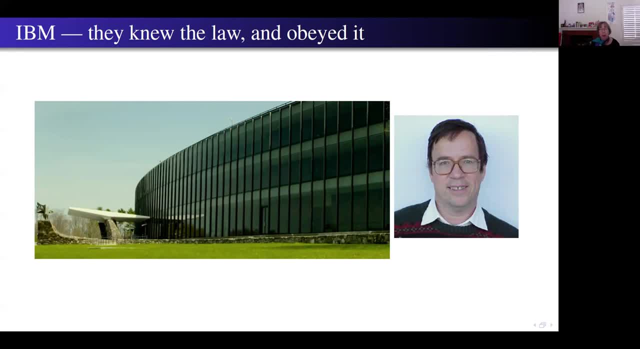 Well, there are a number of stories I can give. I'll just give you a few, So I'll start with one of them. So, before I started at IBM, they asked me what type of computer I used. And I told IBM that I used a Macintosh. So IBM bought me an Apple computer. 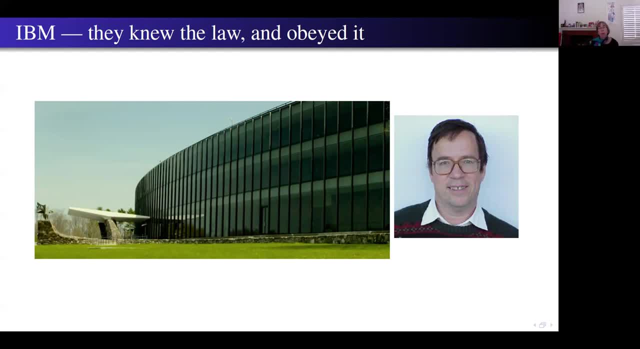 and they bought all the software that I planned to use, even though I already had a lot of the software. So they were real sticklers for the rules, both in paying for software and also in a lot of other ways. And I would tell people that the difference I saw between IBM and academia was: 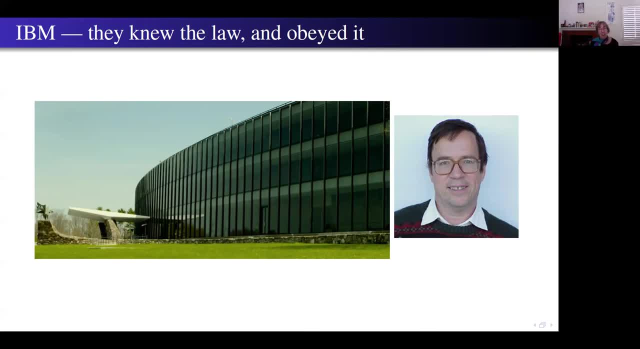 that IBM knew the law and obeyed it. And in fact, when I was in Silicon Valley a decade or so later, I noticed that not all companies were so good about knowing the law and obeying it. So by the turn of the century, Silicon Valley was starting to look like the TV show Silicon Valley. 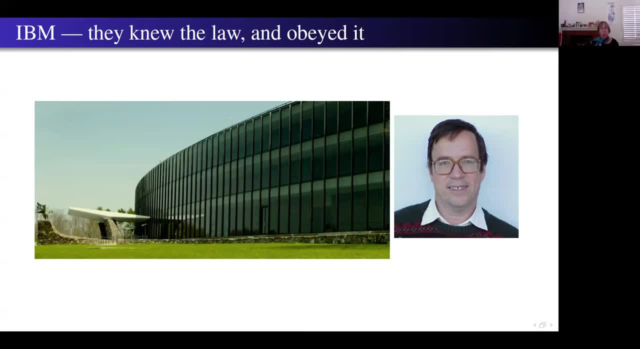 Don Coppersmith's extraordinary abilities as a cryptographer, I think, are well known. So sometime later I was talking with a mathematician about a cryptosystem that person had published, which soon turned out to be broken, And I asked: well, why didn't you run it past Don Coppersmith before? 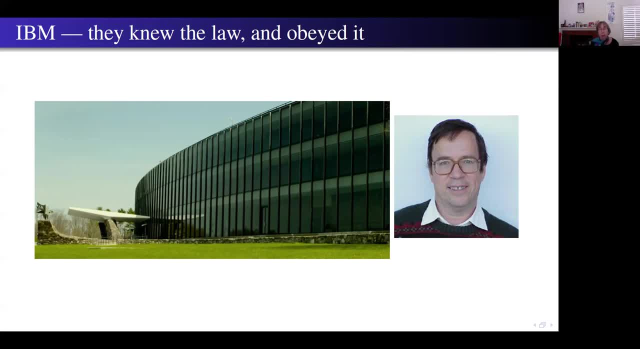 publishing it. And he replied: well, of course I wasn't going to do that. He would have just broken it and I wouldn't have gotten a paper. Well, so it'd be nice if getting things right were more important than publishing a paper. One more IBM story: A computer scientist there had solved a 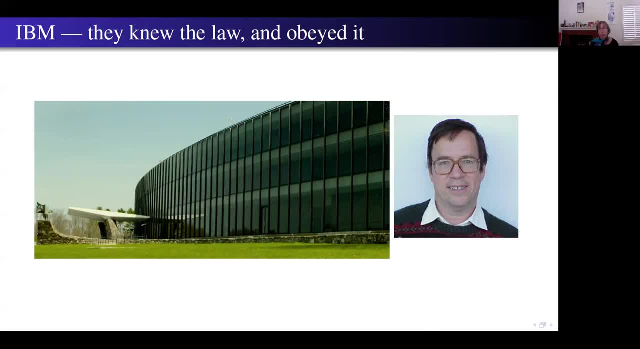 problem by doing an immensely complicated brute force computation, And he asked me if I knew a better way to solve it. So I thought about it and realized that what he wanted falls out immediately from something called the structure theorem for modules over a principal ideal domain. And you don't have to know. 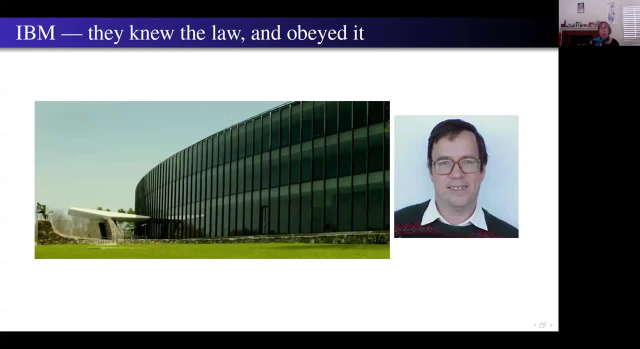 what that means. He was very happy and it shortened the paper considerably, And he wanted me to be a co-author on the paper. Now I was completely horrified because all I had contributed was something that I had learned when I was an undergraduate. So as far as I was concerned, 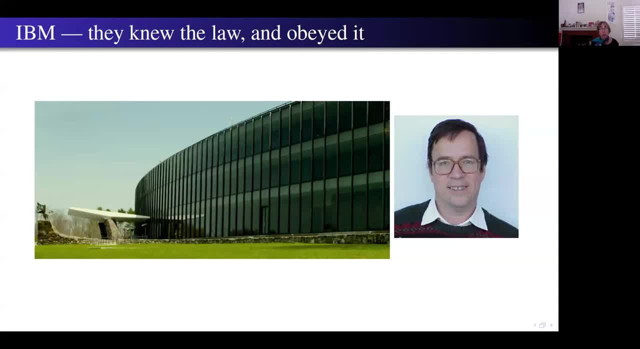 it wasn't at all deep and it would be embarrassing to put my name on the paper Now in retrospect. that was a clear mistake on my part. So the result had applications. It was useful And by working with people in other fields, I hope that I've learned to become 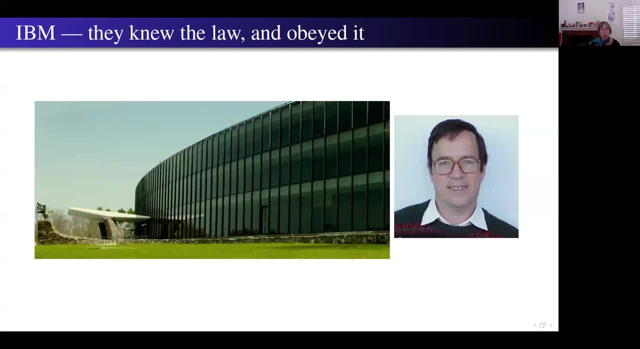 more open-minded. In fact, my most cited paper is one of my least mathematically deep papers. So for mathematicians working with other cryptographers, it can be helpful to know that being deep can be very different from being useful, and being useful can be a good thing. 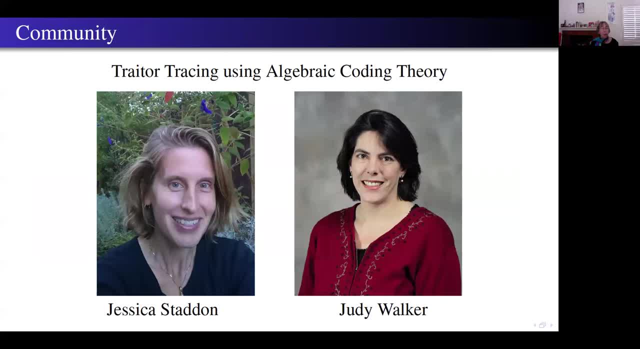 Having a supportive community can be very important. So when I first moved into cryptography research, the cryptography community was very, very supportive and a number of people helped me to make that transition, And I found that particularly young female computer scientists were especially supportive. So in particular, Jessica Stadden invited me to be a visitor at 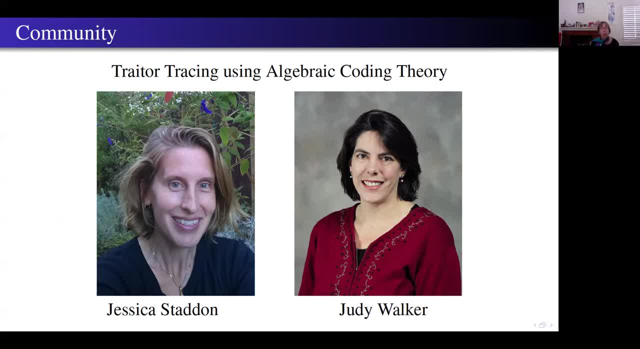 the research labs where she worked and she came up with a problem for us to work on together in trader tracing And she said: well, you know, I'm not a computer scientist, I'm a computer scientist. We soon realized it would be helpful to have an expert in algebraic coding theory in the project. 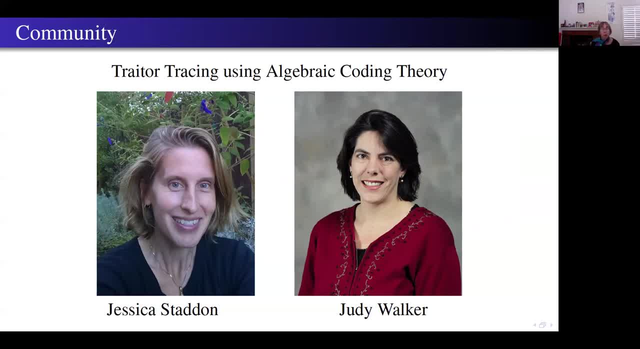 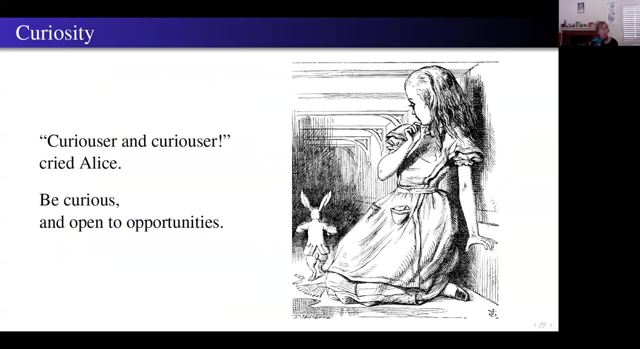 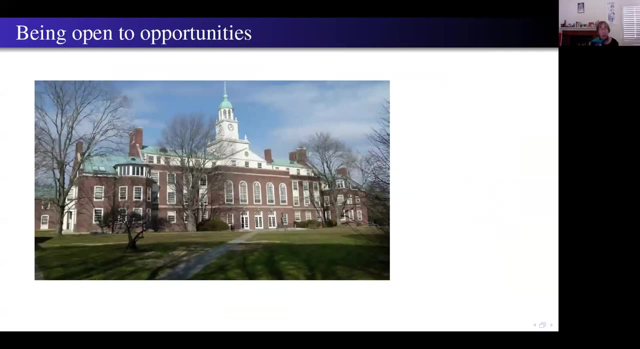 and we were joined by Judy Walker. So I'm a great believer, again, in bringing in experts when one needs specialized expertise. Okay, be curious and open to opportunities. So in the fall of 1995, I was visiting the Institute for Advanced Study in Princeton, New Jersey, And I felt like Cinderella. 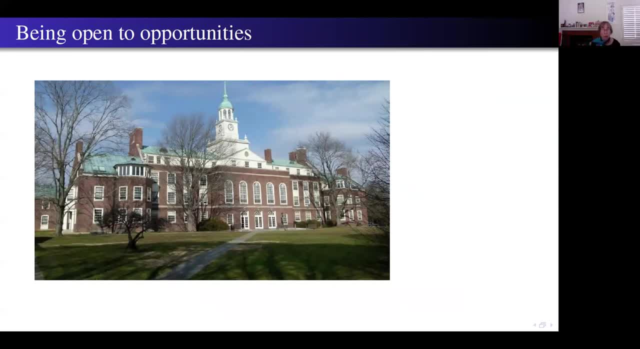 because they put me in a horrid dark room in the attic of Fould Hall with no air conditioning, and I arrived in a sweltering summer. I remember that the cord on the lamp was frayed and I was worried that I was going to get electrocuted. The desk chair fell over backwards, if you lean back. 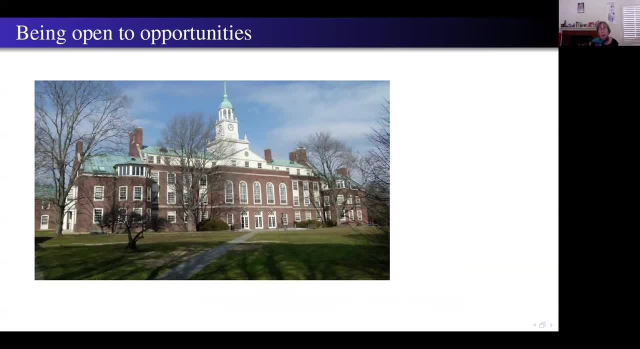 even just a little bit, and the room was almost impossible to find. So I was startled when one day, when I was feeling particularly sorry for myself, there was a knock on the door. So I felt like you know, as Edgar Allan Poe said in the Raven, who's that knocking at my door? 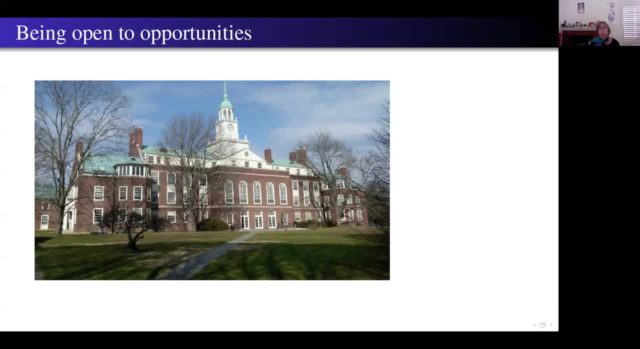 I figured it must be someone who was lost. Well, it turned out to be a grad student in computer science who trekked over from Princeton University and tracked me down to ask me questions about abelian varieties. So this was someone who was curious, open to opportunities and knew that. 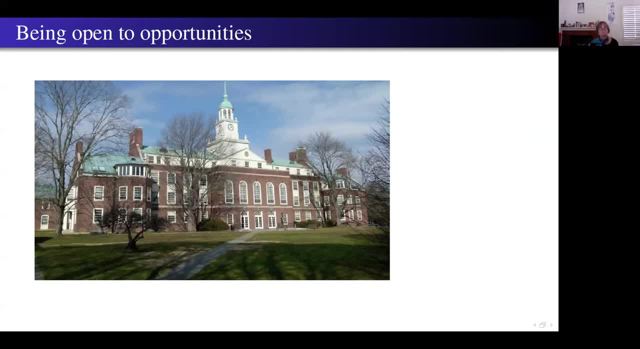 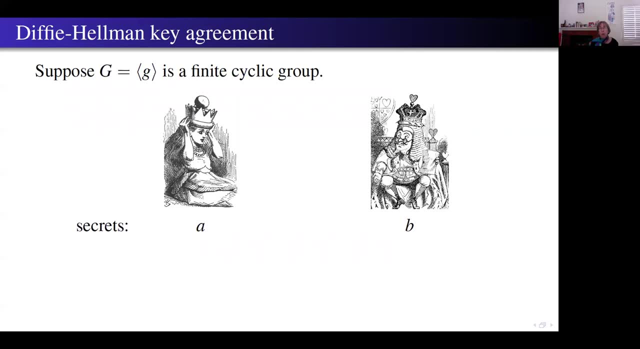 it's worthwhile to talk with a specialist in the field, and that's how I met Dan Boneh, to use Diffie-Hellman Key Agreement as a starting point. Now, if you don't want to hear anything technical, feel free to skip ahead. maybe 10 or 15 minutes- 10 minutes, let's say in this talk. 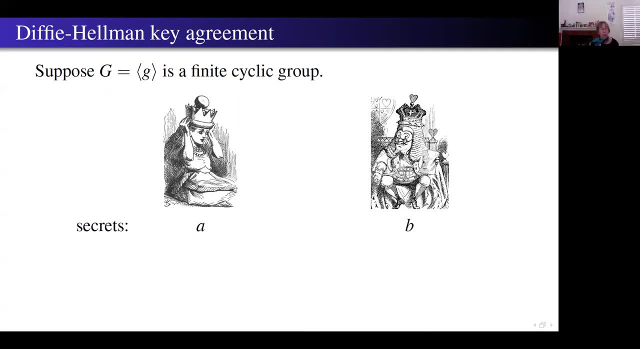 That's fine. Now, at this point, you have a right to complain to me and say jargon, you're using jargon. So this slide starts with: let little g be a generator of a finite cyclic group, capital G. 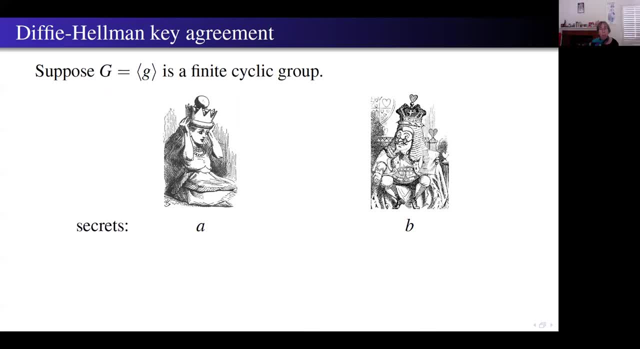 Okay, if you don't know about finite cyclic groups, that's fine. I give you permission to think of little g as an integer, and when I say g to the a, that means take g to the power a and take its remainder and division by a large prime number, Or you can skip ahead in the talk. 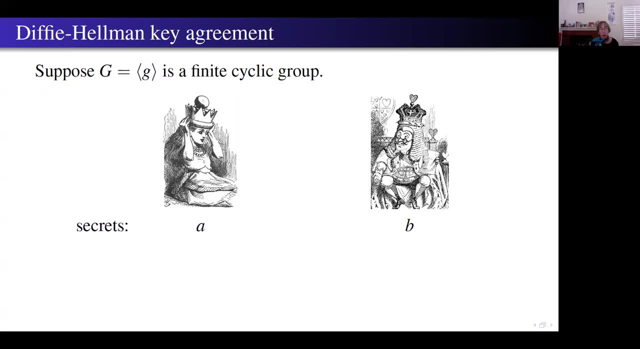 Okay, so Bob and I want to create a shared secret, So we have our own secrets. I have little a, Bob has little b, some numbers integers. I broadcast or send g to the a, Bob sends or broadcasts g to the b and we share g to the ab. 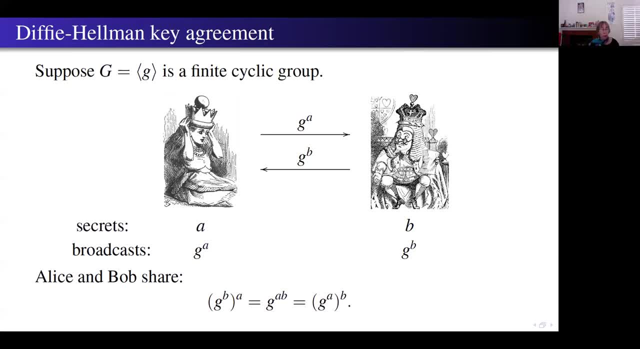 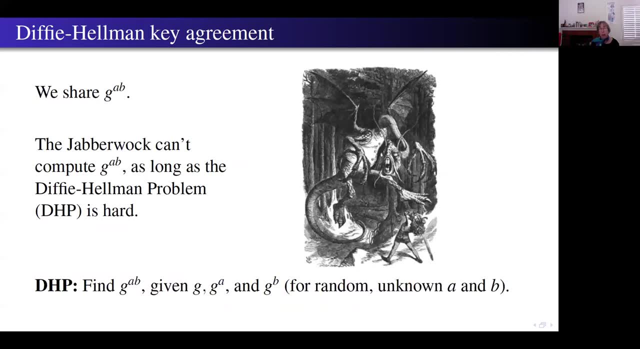 Which we can each compute by taking the broadcast that we've seen and raising to our secret number, And we both get g to the ab that way. So we share that value And I claim that nobody else knows that value. So why can't the adversary compute g to the ab? Well, the adversary in this case, 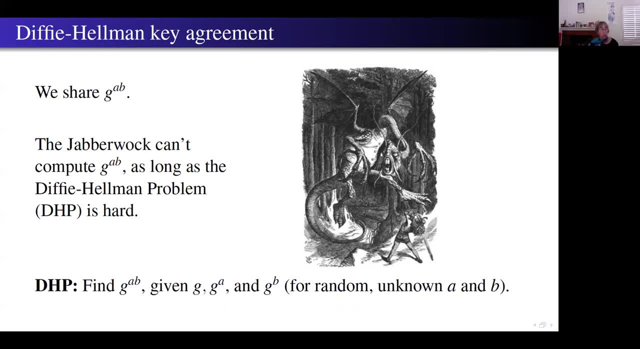 the jabberwock can't compute g to the ab as long as the Diffie-Hellman problem is hard. where the Diffie-Hellman problem is the problem, the answer is g to the ab, given g to the a and g to the b for random unknown integers a and b in a certain interval. 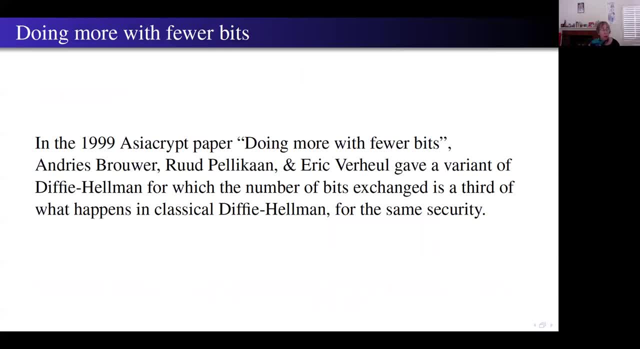 Okay. In a paper in 1999 that appeared in Asia Crypt called Doing More with Fewer Bits, Brauer, Pelikan and Verhul gave a variant of Diffie-Hellman that did more with fewer bits. So the number of bits exchanged was a third of what happened in classical Diffie-Hellman for the same security. 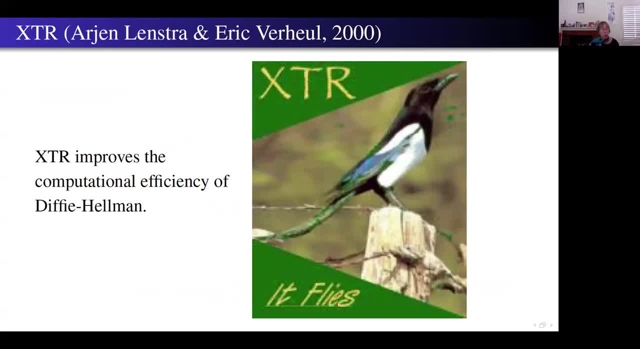 Shortly after that, Arien Leinster and Eric Verhul came up with the XTR cryptosystem, which was an improvement on Brouwer Peloton Verhul. So here is XTR, it flies and they used a magpie. 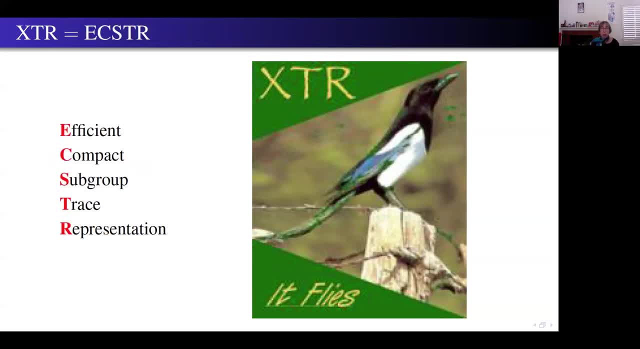 So why a magpie? Well, the X, of course, is short for ECS. So this is now EXTER. EXTER is the Dutch word for magpie And EXTR stands for Efficient Compact Subgroup Trace Representation, Or does it? 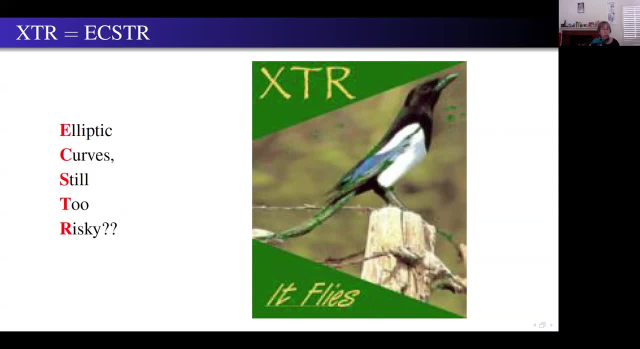 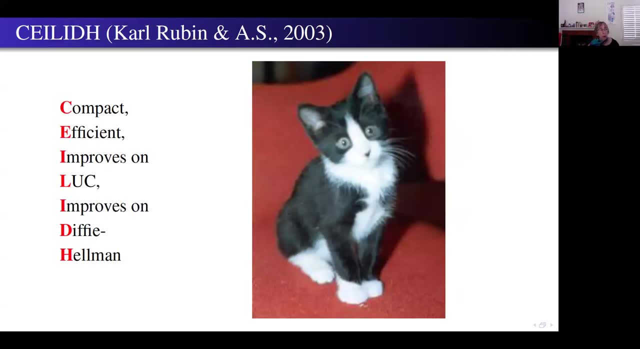 So their joke version was that it stands for Elliptic Curve, Still Too Risky, which, as an elliptic curves person, I found well interesting. Well, a few years later, Carl Rubin and I came up with the Cayley cryptosystem, which 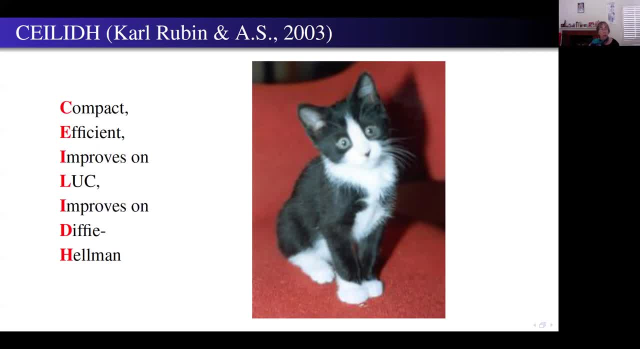 we named after my cat, Cayley. Now, if you have a cat named Cayley, now I use the Scots Gaelic spelling for Cayley- If I use the Irish spelling, it's Cayley. If I use the English spelling, it wouldn't have had the D-H, so it wouldn't have had. 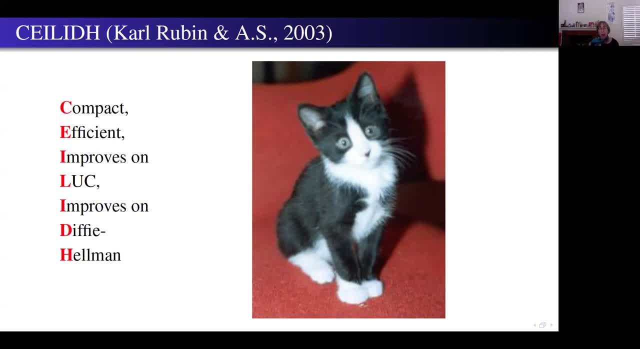 the Diffie-Hellman at the end, But if you have the D-H at the end, it's crying out to be an acronym for something with Diffie-Hellman in it. So the Cayley cryptosystem is compact, efficient, improves on Luke, so Luke can be viewed as: 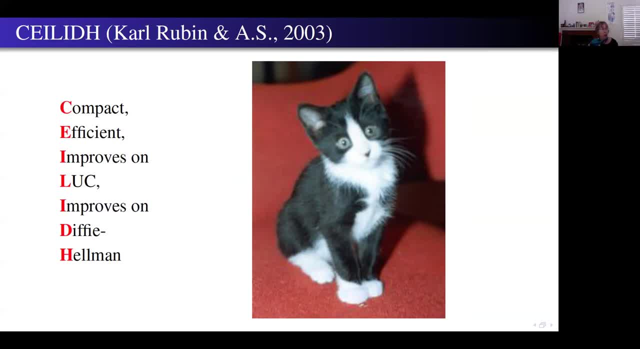 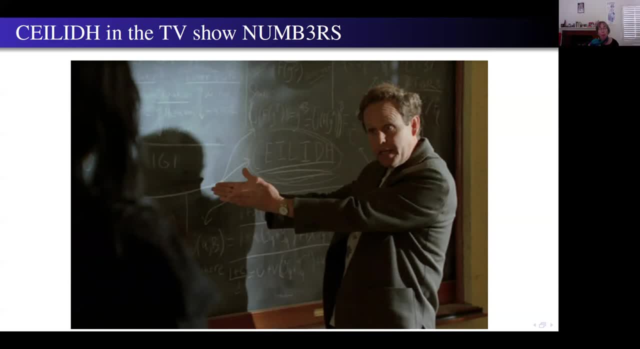 a forerunner of XTR. it was a Luka-based cryptosystem and improves on Diffie-Hellman, And I was a consultant for the television show Numbers. It's a wonderful thing about being in cryptography: you can come up with these cute names and 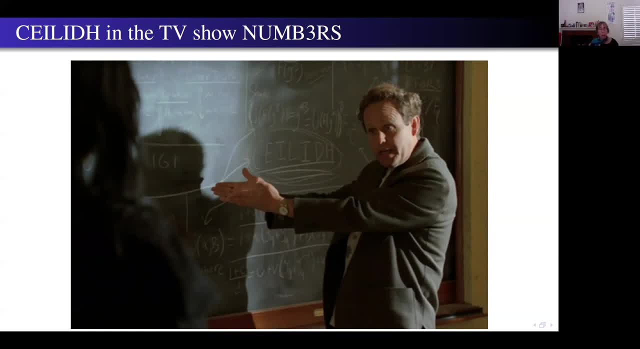 put them in the background of the scene And in one episode they had something on cryptography and they asked me for something to put on the blackboard to have in the background of the scene. So I gave them the equations for the Cayley cryptosystem. 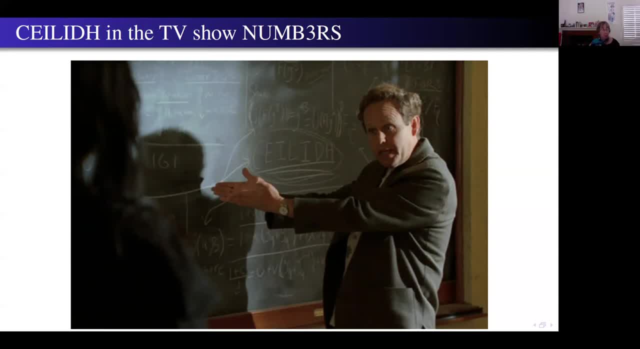 And here you can see the word Cayley in the middle of this slide, and the equations for the Cayley cryptosystem are all around it. So when that aired, over 12 million viewers saw the name of my cat, Cayley, flash across. 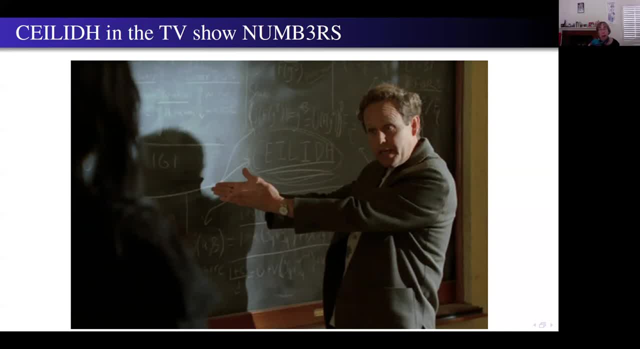 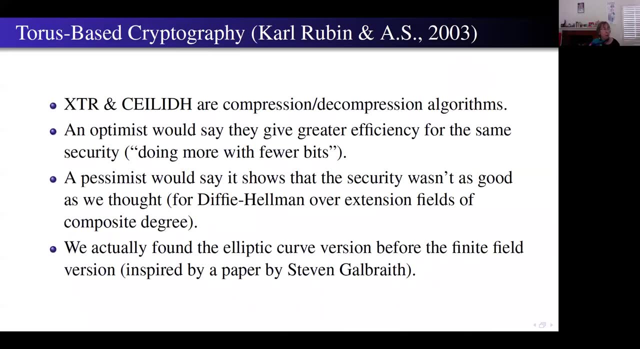 their TV screens, which is probably about maybe 12 million times the number of people who would ordinarily read one of my math papers. Okay, well, we also came up with a mathematical explanation for what was really behind the Luka-based cryptosystems in XTR and Cayley, and we called that Taurus-based cryptography. 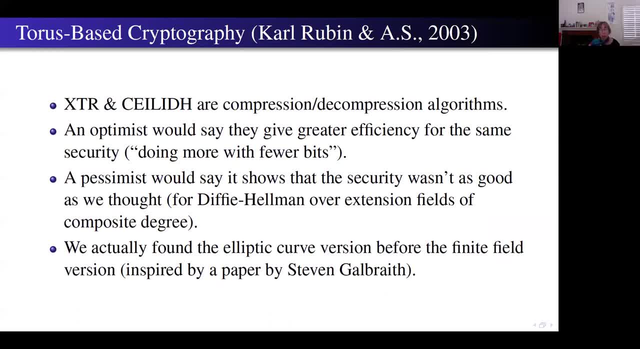 because it relied on the mathematics of something called algebraic tori, not to be confused with complex tori that some of you know from elliptic curve theory. So Luka, XTR and Cayley can be viewed as compression and decompression algorithms. 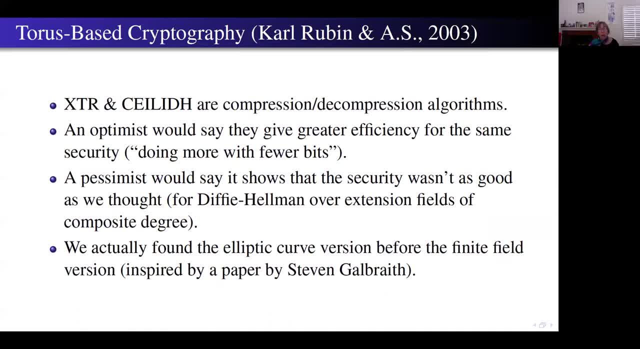 So you might say that they do more with fewer bits. Now, what a couple of people pointed out to me is that there's a flip side to that, which is that if you're not, if you're only using some of the bits, then those other bits weren't. 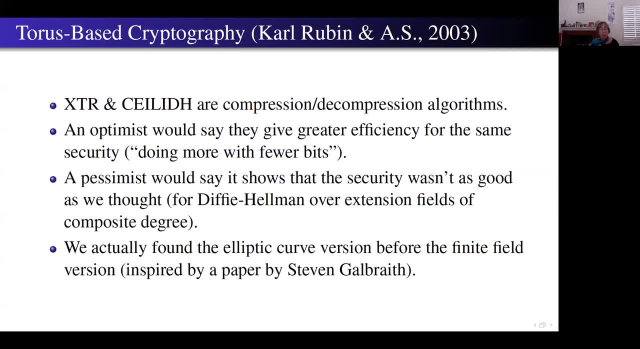 really giving you security. So in some sense it's telling you that maybe the security that you thought you had you didn't really have. The security wasn't as good as we thought. Now this doesn't have an effect on the security of Diffie-Hellman over prime fields, but it's. 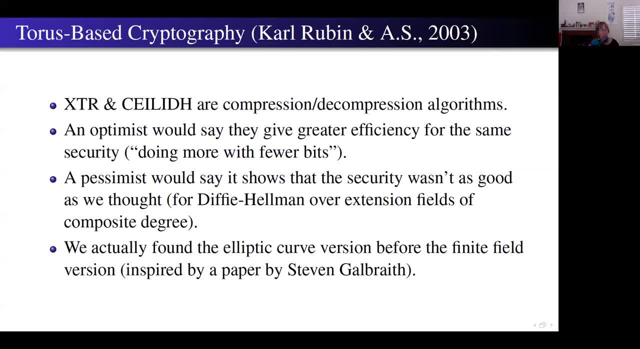 somewhat relevant for Diffie-Hellman- over extension, fields of composite degree And, interestingly, usually in public key cryptography. if you have something over finite fields, then there's an analog for elliptic curves. that usually comes later. In this case, actually, the elliptic curve version came first. 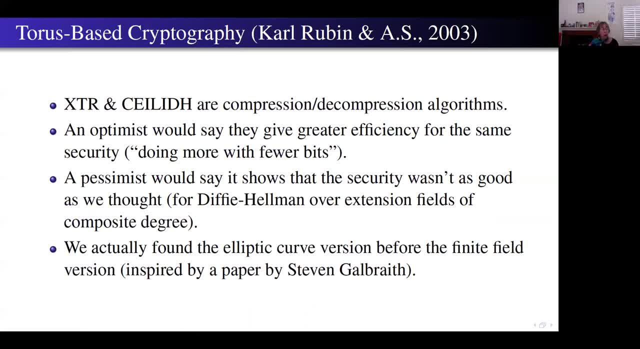 So the finite field version is the torus-based cryptography. We had an elliptic curve or abelian varieties version that was inspired by a paper of Stephen Galbraith on super singular abelian varieties in cryptography. Okay, what if three parties want to create a shared secret? 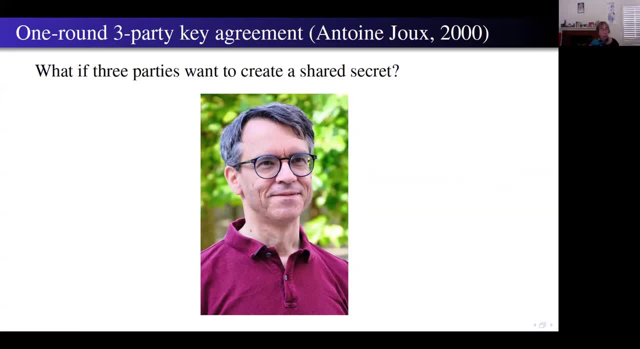 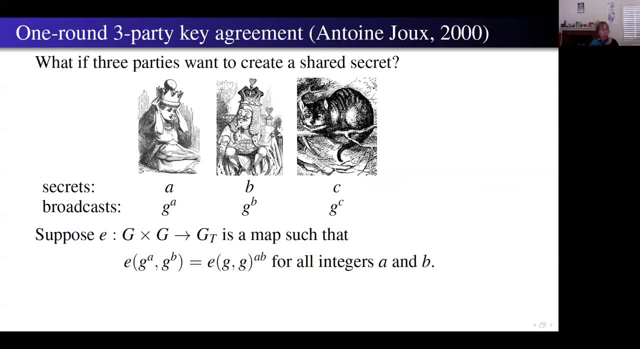 Well, that was solved by Antoine Jou in a paper in the year 2000.. So the three of us each have our own private secrets, we have our broadcasts and if we have a map that takes two inputs and has this bilinearity property, so if we take two elements, 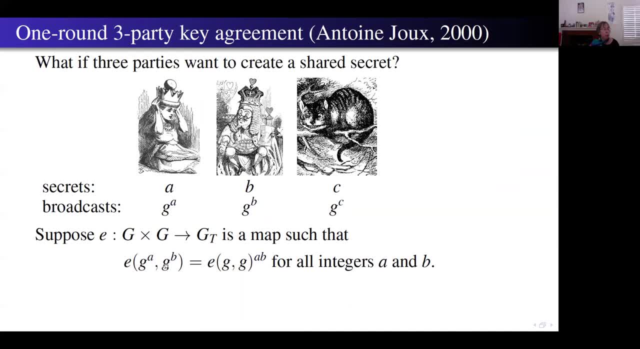 of our group, g to the a and g to the b, and those are our two inputs into the function. if what we get is the same as what you get when you input g and g, take the output and raise it to the power ab, so I'm going to call that the bilinearity property, if you. 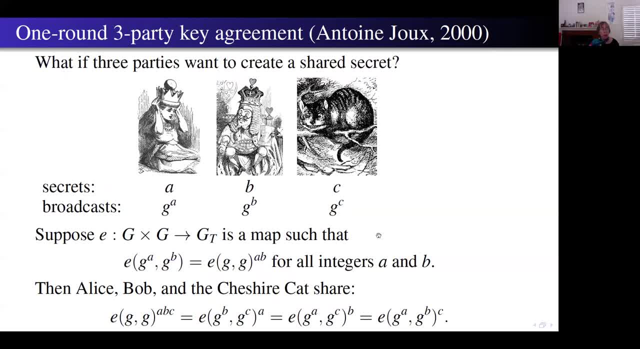 have that bilinearity property, then Bob the Cheshire Cat and I are going to be able to create a shared secret. Okay, So I have something that we can all compute. we have a shared secret, and it's this thing what happens when you input g and g and then take the output, raise it to the power abc. 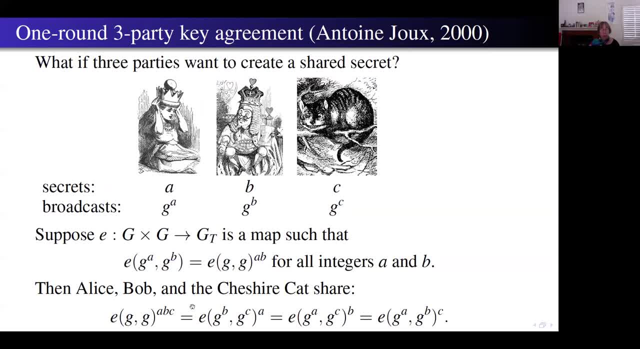 which we can each compute by taking the two broadcasts that we receive, inputting those into the function and raising to our secret power. and that's because of the bilinearity property, which says that you can pull out the exponents and get this. 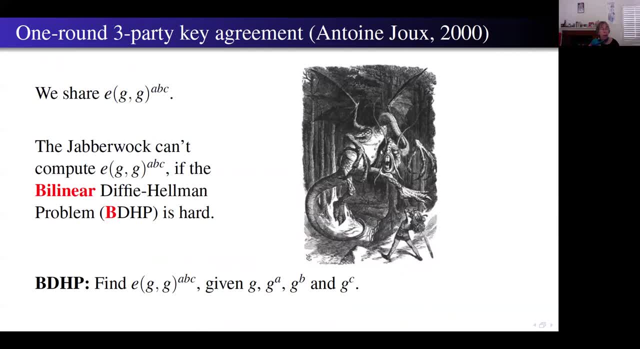 Okay, so we share this value. why can't the java walk compute it? The java walk cannot compute it if the bilinearity Diffie-Hellman problem is hard. where the bilinearity Diffie-Hellman problem says: find the supposed secret information, given the 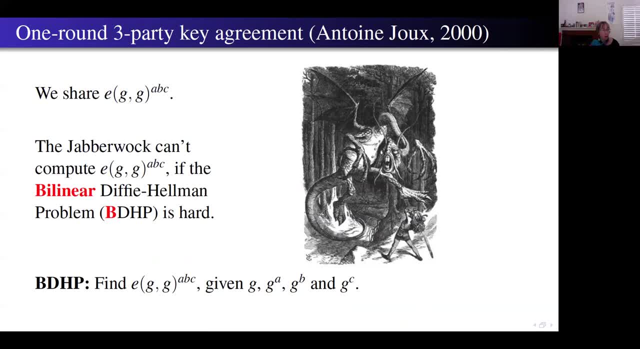 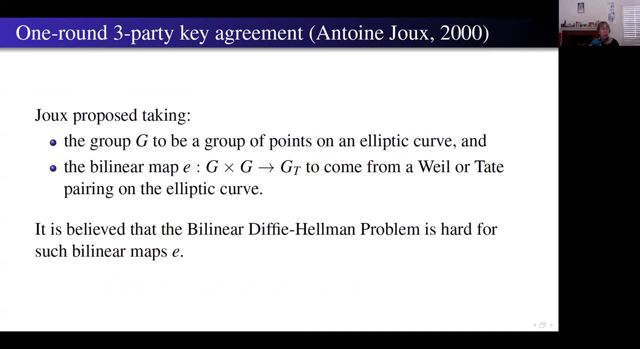 public information. So it's basically a tautology that the security depends on the bilinearity Diffie-Hellman problem And Antoine Jou, when he proposed this, proposed using taking the group to be the group of points on an elliptic curve and taking the bilinear map to be a map coming from a they. 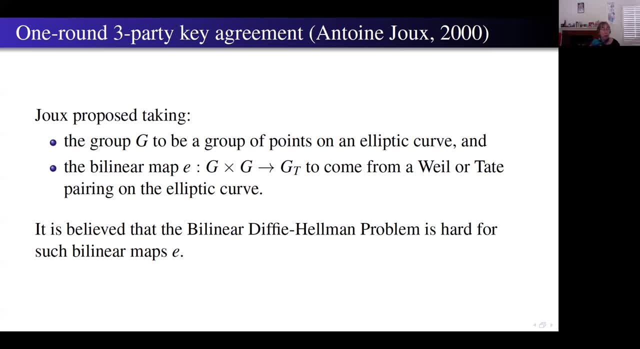 pairing, or a they pairing, on an elliptic curve And it's believed the bilinearity Diffie-Hellman problem is hard in that setting And I'll say that they pairings had been around for a long time and were well known to number. 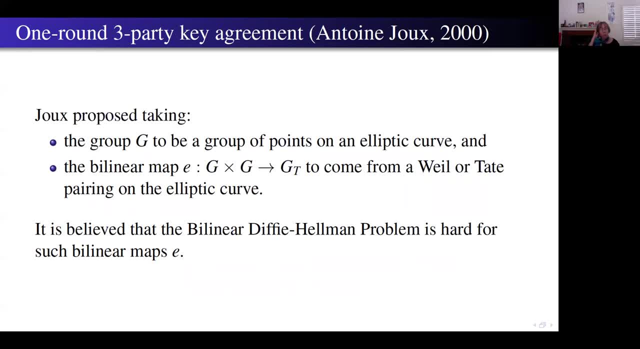 theorists in the field, number theorists who look at elliptic curves, and perhaps if more mathematicians had been involved more heavily in cryptography, some of this might have happened sooner. I will say that a decade earlier, pairings on elliptic curves were used in a destructive 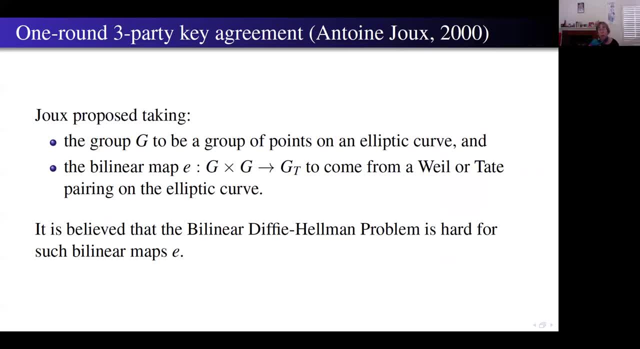 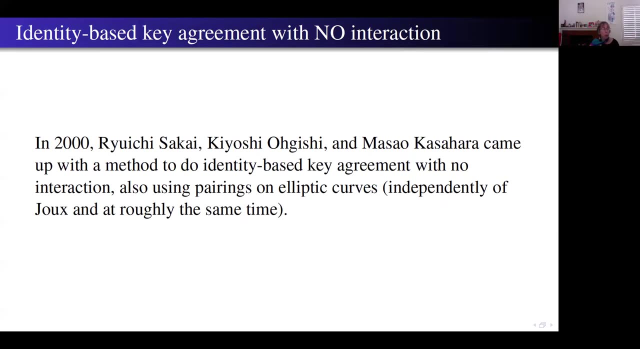 way. The MOV attack due to Menezes, Okamoto and Vanstone was a way to attack the decisional Diffie-Hellman problem, But then it took another 10 years to use it in a constructive way. And at the same time, also in 2000,, Sakai Ogishi and Kasahara came up independently. 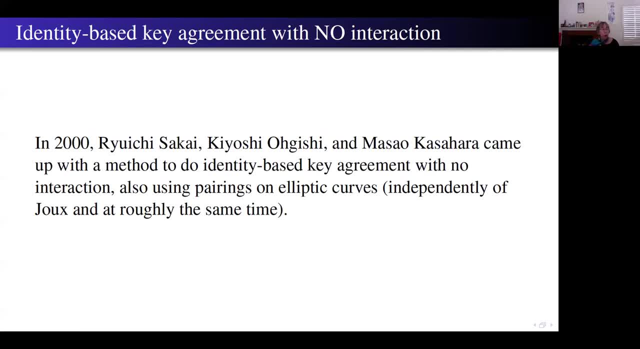 with a method to do identity-based key agreement with no interaction, Also using pairings and elliptic curves, so actually no broadcasts, And so that was the origins of pairing-based cryptography. can be viewed as those two papers from the year 2000,. Sakai Ogishi Kasahara and Antoine Jue's paper. 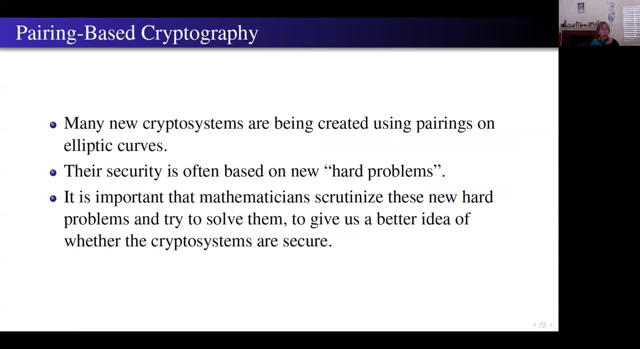 So after that there were many new cryptosystems that were created using pairings and elliptic curves. Their security was often based on new hard problems. so in addition to bilinearity- Diffie-Hellman, often one had to come up with other problems that were presumed to be hard and the security 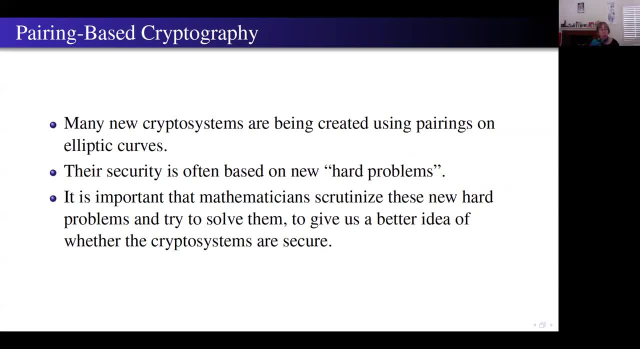 of the new systems were based on them. So it's important for mathematicians to scrutinize these new hard problems- because they're basically number theory problems in some sense- and try to solve them so that we have a better idea of whether these cryptosystems are actually secure. 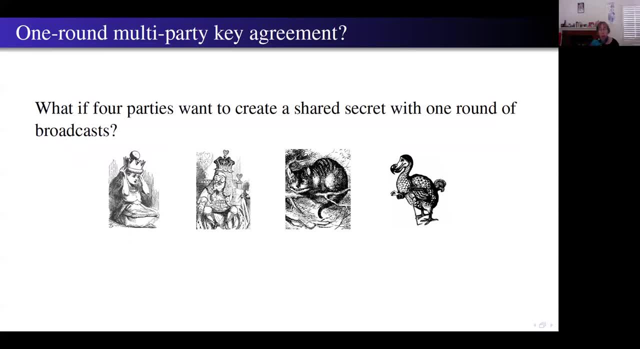 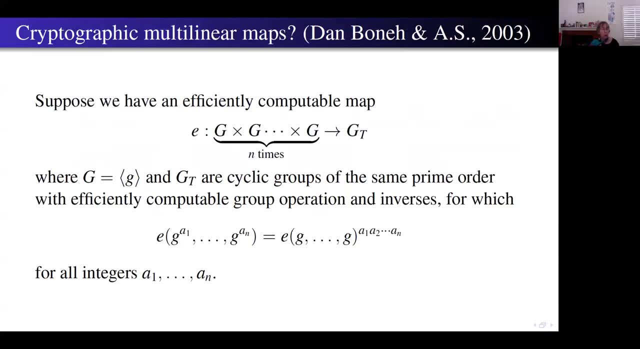 Okay, what if four parties want to create a shared secret with one round of broadcast? Well, open question. So Dan Bonnet and I considered that question in a paper that appeared in 2003.. We said that if you have a function where, instead of the bilinearity property and instead 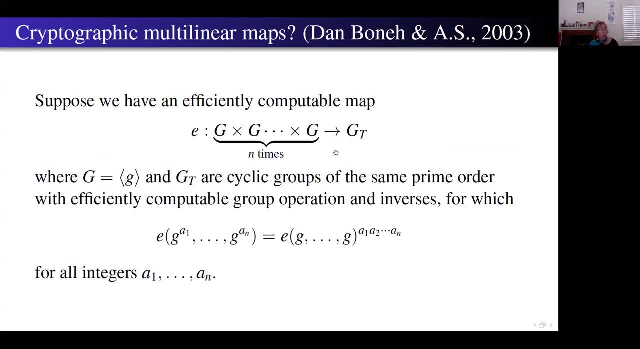 of having two inputs. you have n inputs and you have this. you replace bilinearity with multilinearity, so it's a direct generalization. so you have your n inputs coming from your group. your inputs are g to the power a1 up to g to the power an and you want the value. 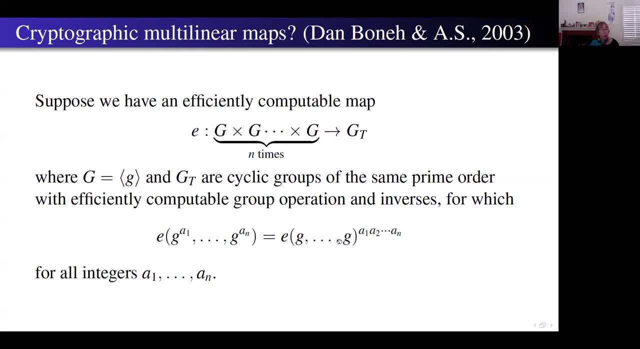 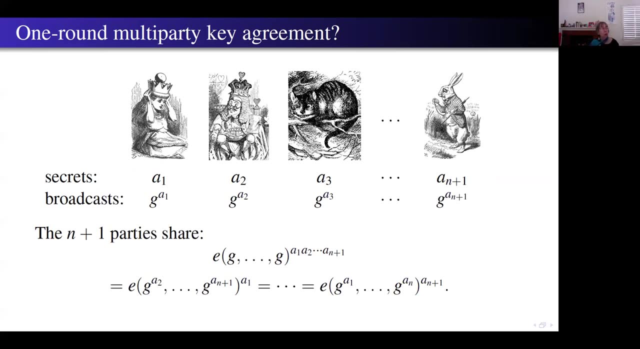 that you get when you input those To be the same as if you inputted g n times, took the output and raised it to this product product of a1 up through an. So that's the multilinearity property. So if you had such a function then n plus one parties could create a shared secret key. 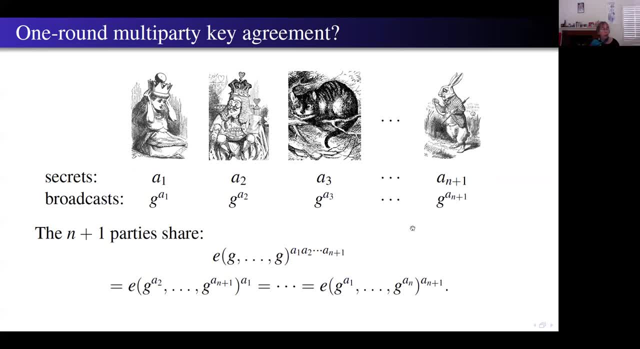 So we have our secrets, we have our broadcasts and I claim we share this value. The way we each compute it is: we take the n broadcasts that we see. Those are our n inputs to our n-valued function, to our function with n inputs. 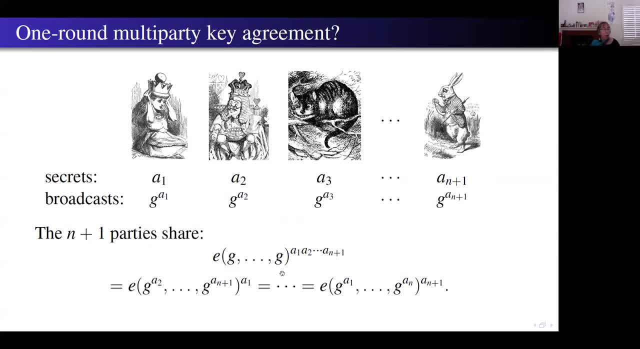 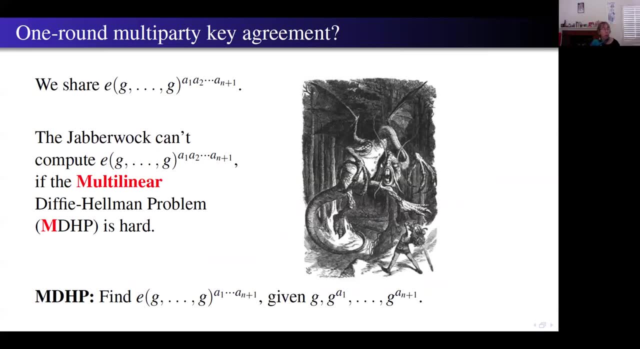 We take the output, we raise it to our own secret and by the multilinearity property we all get the same value. And the reason it's secure, the reason the Jabberwock doesn't know this value. well, it's secure if the multilinear Diffie-Hellman problem is a hard problem. 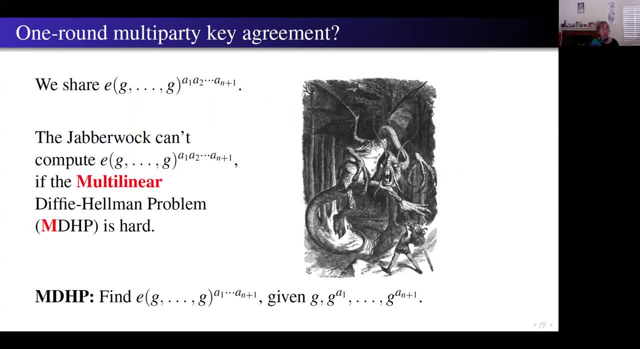 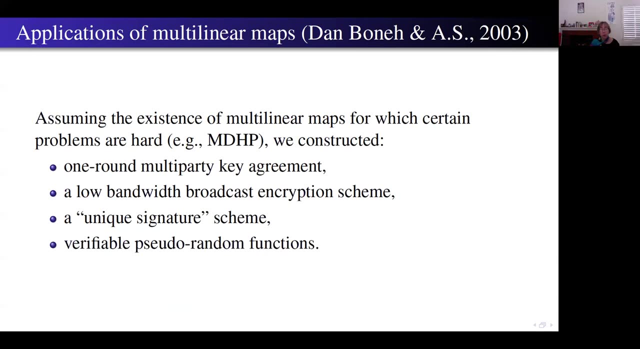 So what's the multilinear Diffie-Hellman problem, say? Well, surprise, surprise, It says that it's. It's the problem of finding the secret information, the shared information, given the public information. So, assuming the existence of such multilinear maps which we didn't know how to construct, 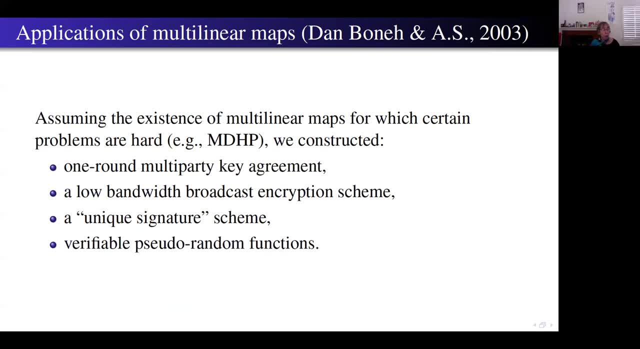 if you have more than two inputs, we could construct all sorts of nice things, But we might have. We had to add some other hard problems, some other problems that we hoped were hard problems in some cases, not just the multilinearity Diffie-Hellman problem. 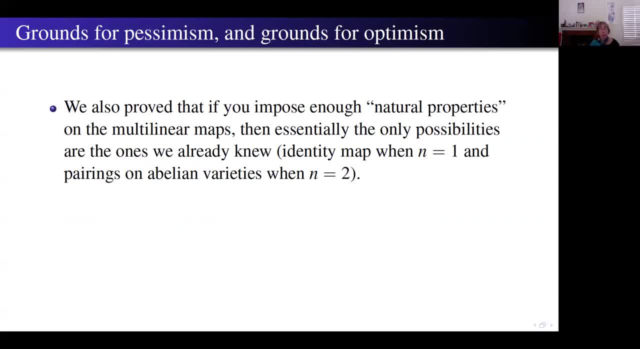 But there's a dark side to our paper, and the dark side is: well, the Weil pairing has lots of lovely properties, lovely from a mathematician's point of view. So it has these very natural properties. and if you impose enough of these properties on, 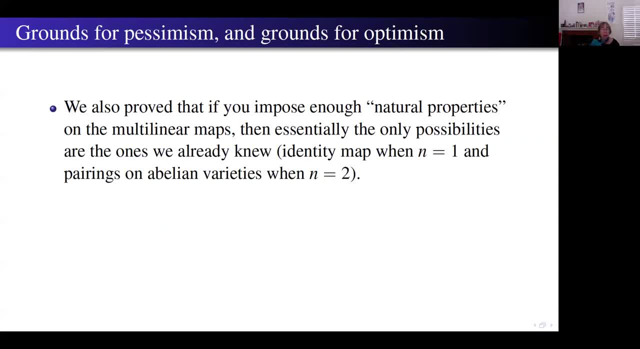 your multilinear maps, then we can prove that you're not going to end up with anything really other than a variant of something you already knew. So in the case when n equals one, you have the identity map. That's classical Diffie-Hellman. 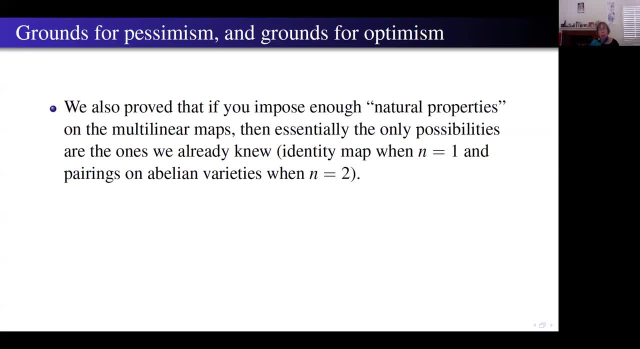 When you have two inputs, you have pairings on elliptic curves or abelian varieties. That's pairing-based cryptography and that would be basically all you would get. But the good news is that, as people were doing pairing-based cryptography, they came up with 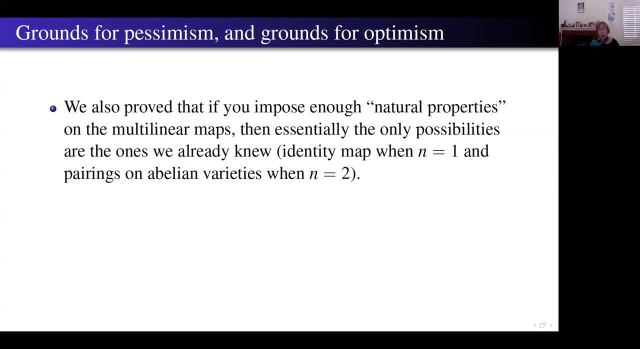 more and more pairings that were useful to use, that were efficient and seemed to work well, and they didn't necessarily have mathematically natural properties. They didn't make mathematicians cringe in some cases, but they were useful. So being mathematically beautiful isn't necessarily the right criterion to use. 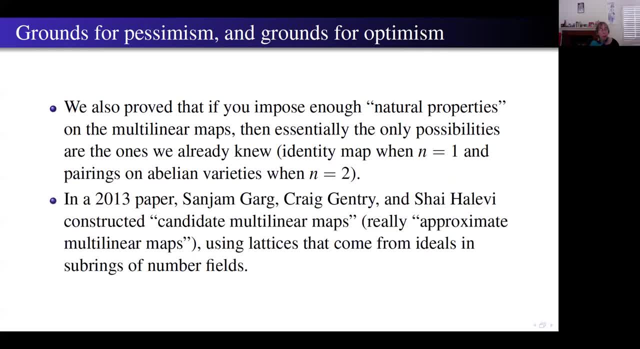 Being useful is perhaps more important, And another good sign was that in 2013,, Garg, Gentry and Halevy constructed what they called candidate multilinear maps, and I think of it as approximate multilinear maps, So they didn't fall strictly within the framework that Dan and I had envisioned. 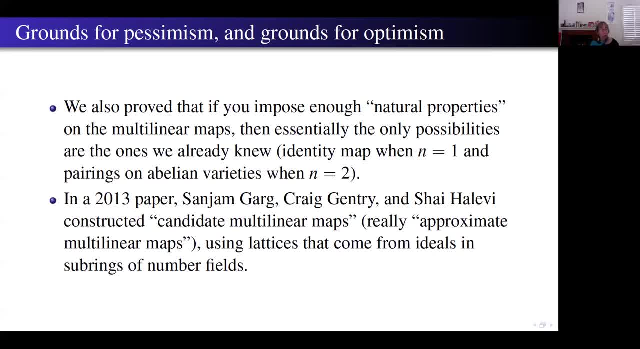 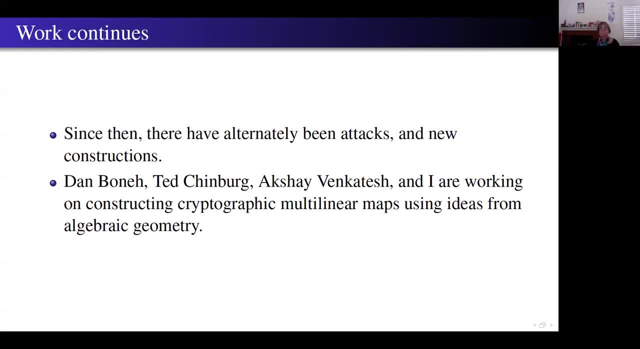 But But they, you know they're useful. It seemed like they would be useful And they were constructed using lattices that come from number theory, And since then there have alternately been attacks and new constructions, And there are a number of. 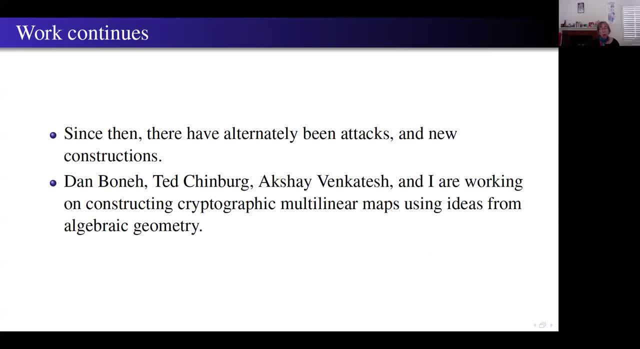 Well, I'd say it's still an open problem to come up with multilinear maps when you have more than two inputs And one. There are a number of groups working on this. One group consists of me and Dan Binet, Ted Kinberg, Akshay Venkatesh, where we're trying. 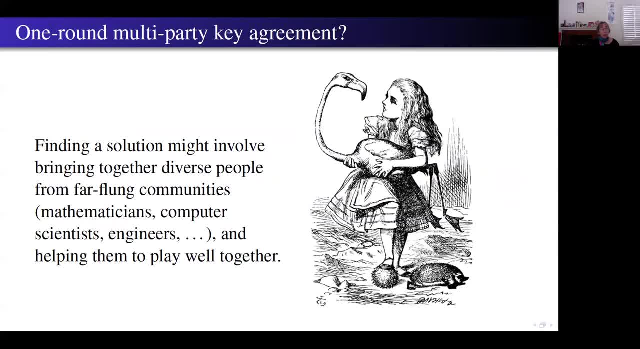 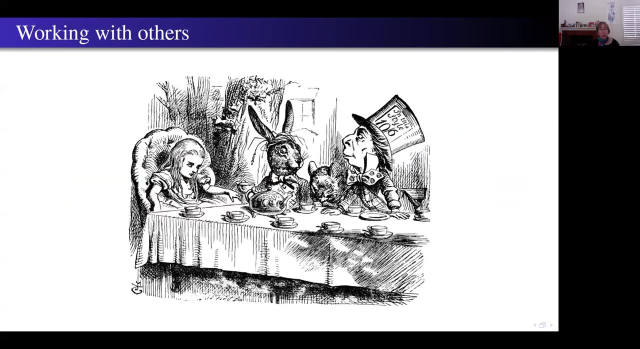 to use ideas from algebra To break geometry. Finding a solution might involve bringing together diverse groups of people, like in our group, from far-flung communities of mathematicians, computer scientists, engineers- and helping them to play well together, So working with others. 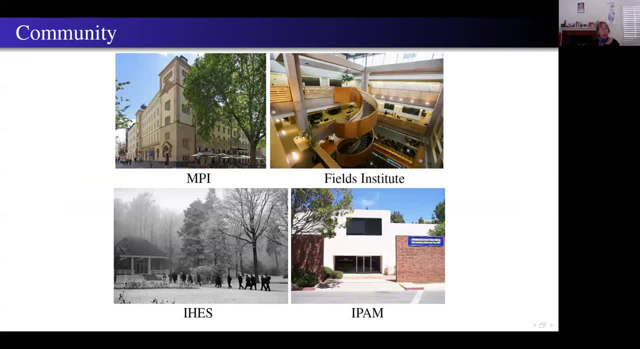 Well, so I mentioned community. Now, the first semester-long programs in cryptography that I remember were in the fall of 2006.. There were two competing programs, one at IPAM in Los Angeles and one at the Fields Institute in Toronto, And I think they happened at the same time because of a failure of communication. 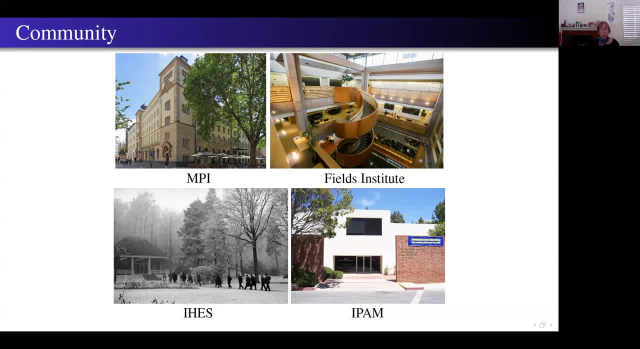 And in the end, most of the mathematicians went to the Fields Institute and most of the computer scientists went to IPAM. And I went to IPAM partly because it was near home, but also mostly because I wanted to interact with computer scientists. 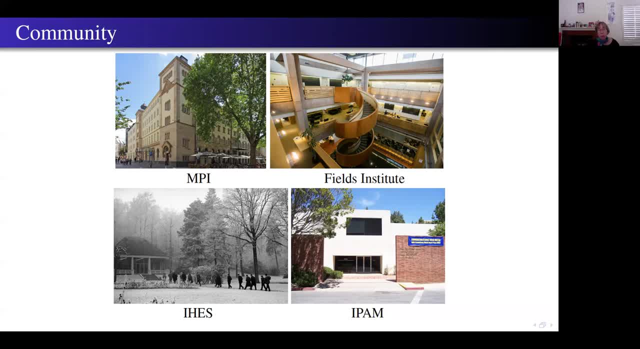 But I did find that many days it felt as if I was the only one there. So it was quiet and peaceful, especially in the evenings, but there wasn't the sense of community that I had experienced at math programs at other research institutes. So it used to be the case that if you were, say, a senior mathematician who was given 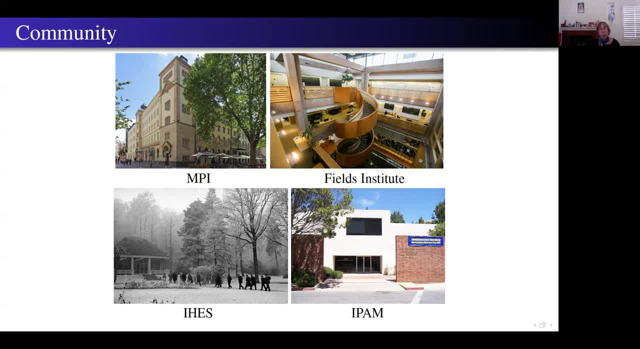 funding to attend a math conference, you felt an obligation to attend the entire conference and interact with junior colleagues and make yourself generally useful and available. And if you were invited to a semester-long program, you were given the opportunity to do that. And if you were invited to a semester-long program, you tried to come for as much as 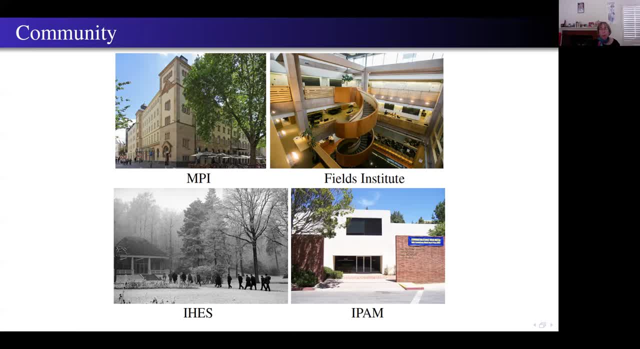 you could of the semester-long program and show up at lectures. Now for cryptography conferences and I think increasingly at math conferences, it's accepted that people might fly in just before their own talk and leave soon after it and only talk with their collaborators. 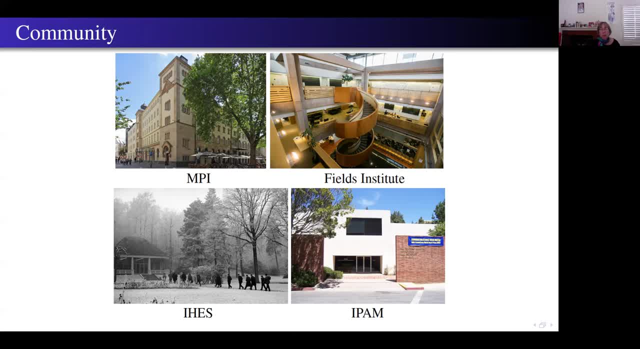 Now I think that maybe the people who say we have too many conferences and it's better for the environment if we didn't travel so much have a point, not to mention that we may not be able to travel for a while, So maybe fewer conferences. 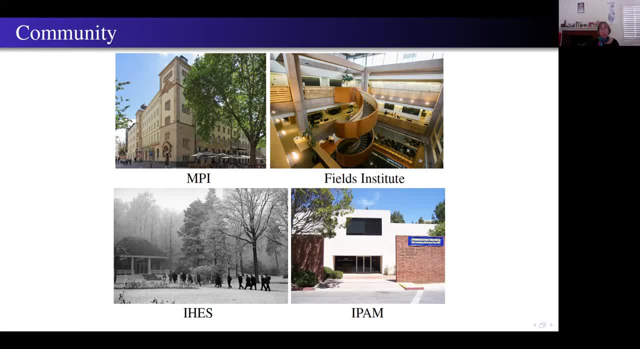 But once we start having them again, stay at them longer, Build a sense of community. So I think it's useful to have semester-long programs with week-long workshops, as a lot of these institutes have, so that people who can't stay for the full program can still. 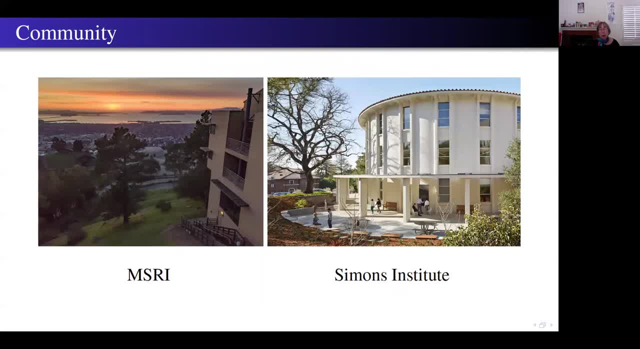 attend some of the workshops. Now, things have changed over time, So this semester I was visiting the Simons Institute for the Theory of Computing at Berkeley, where I'm supposed to be for the whole semester, And I would say they're truly wonderful. There truly was a sense of community there. 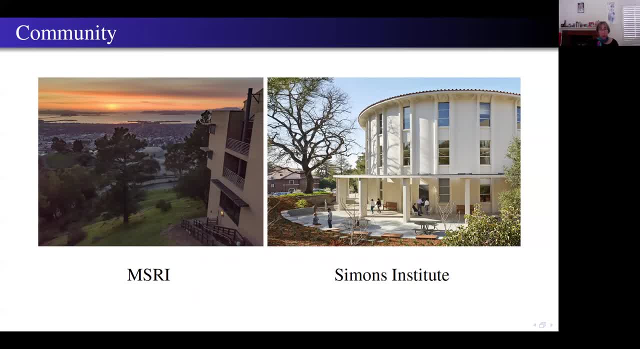 And in fact, when the Bay Area went on lockdown halfway through the semester and everything closed down, it was kind of amazing that that sense of community has continued. So not only did the lectures and workshops go online, which is something the Simons Institute 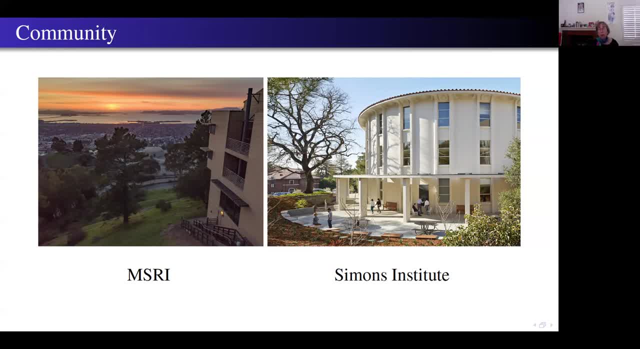 was already very good at doing, but so did the board game night, And new social activities sprang up, like an online cooking class of all things, And I wanted to thank Shafi Goldwasser And the staff for creating and maintaining that really good sense of community. 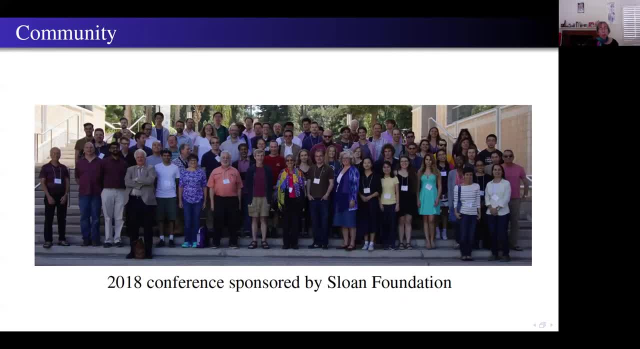 So I've been running a series of conferences and workshops to bring together computer scientists and mathematicians to work on cryptography problems of common interest and especially questions on fully homomorphic encryption and questions about multilinear maps, And I've learned a lot about how to get people from the different communities to work together. 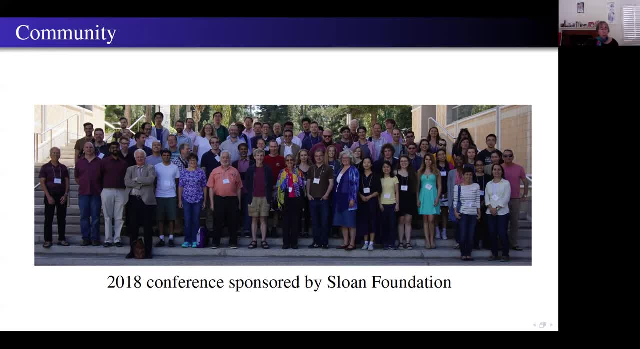 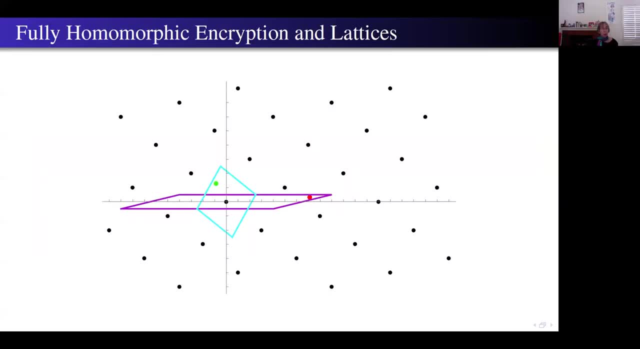 well and to be able to solve problems together, And that's partly me, Thank you. The things that I'm telling you here are often things I've learned from that. I wanted to tell you the story about how I started working on lattice-based cryptography. 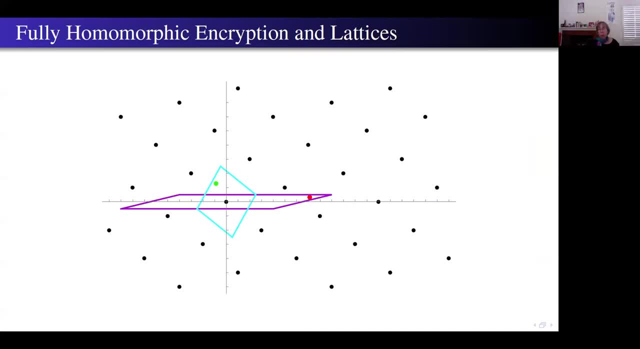 So in the spring of 2011,, I learned about a DARPA initiative on fully homomorphic encryption. Now the DARPA program had already started and there were all sorts of interesting and fun people who were on board already. Now I looked up the call for proposals. 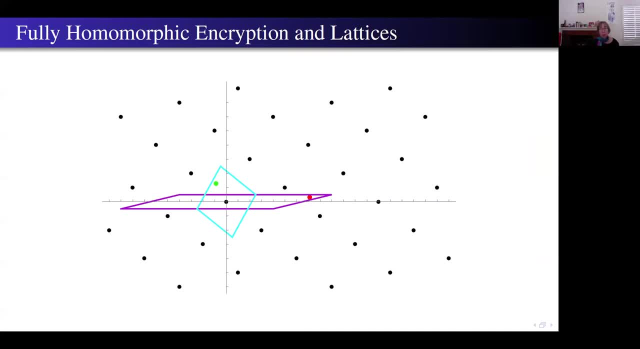 And it has strongly emphasized the message. It emphasized the mathematical foundations And I asked around and it turned out that there were no mathematicians on the project who were working on the mathematics. So I thought, well, I'm someone with a strong math background and I have experience working 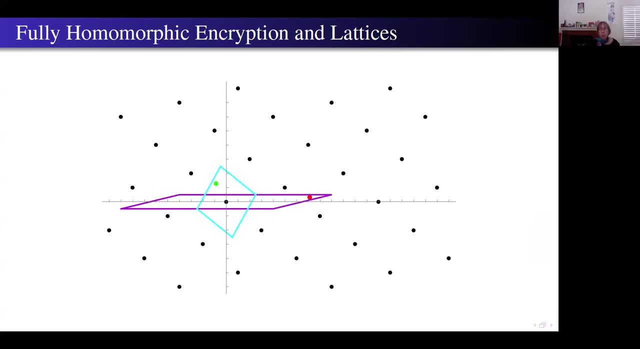 with cryptographers. So I thought to myself I should be on this project. But then it dawned on me that the mathematics of fully homomorphic encryption is lattices, And at that time I didn't know a lot about lattices. 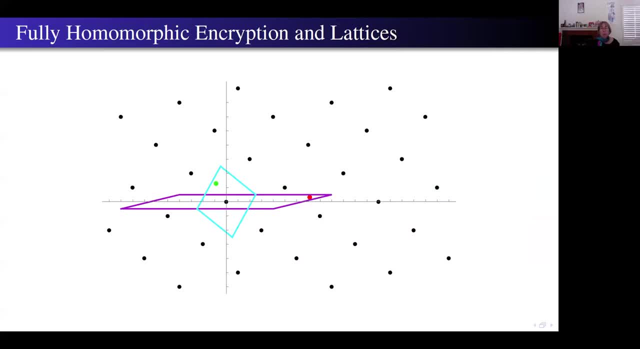 But remember, I'm someone who believes in bringing in the experts And I was visiting the Mathematical Sciences Research Institute in Berkeley and Hendrik Leinster was also there And he's an expert on lattices. So I started bugging Hendrik with questions and we made progress on some problems and 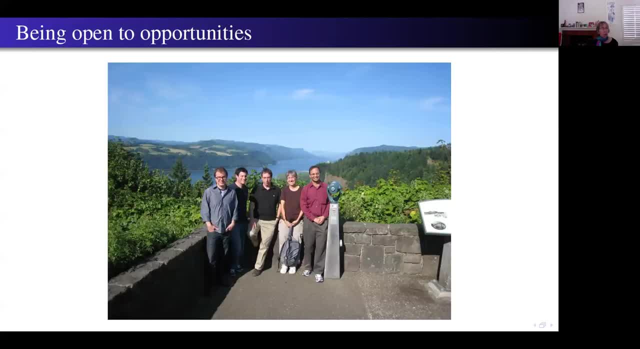 I ended up being added to the DARPA project, So they'd actually run out of money. But mathematicians are cheap. It's easy to add another mathematician or add a mathematician, And it also had the nice advantage that the meeting was very short. 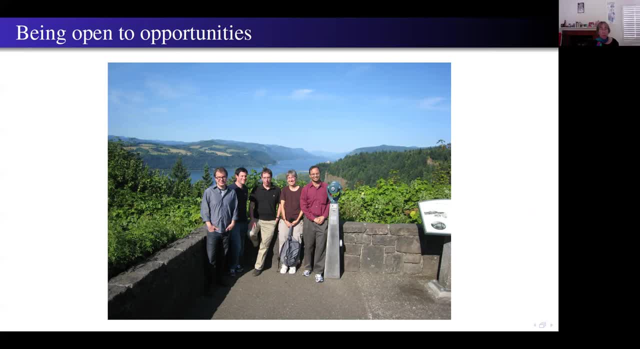 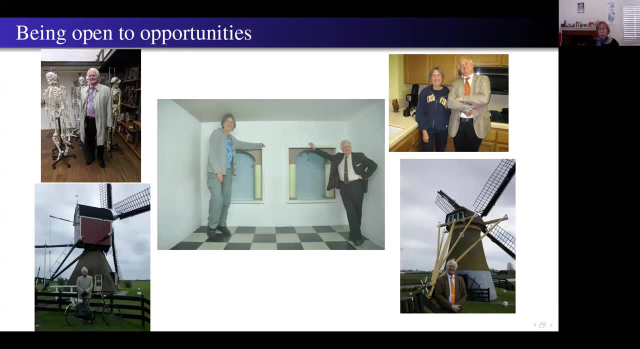 So I was able to do it. The meetings were often in very nice locations, So Hendrik and I proposed using certain lattices with nearly orthogonal bases for fully homomorphic encryption in order to get more efficient decryption. And at some point, Daniela Micentio reminded us about an algorithm of Craig Gentry and 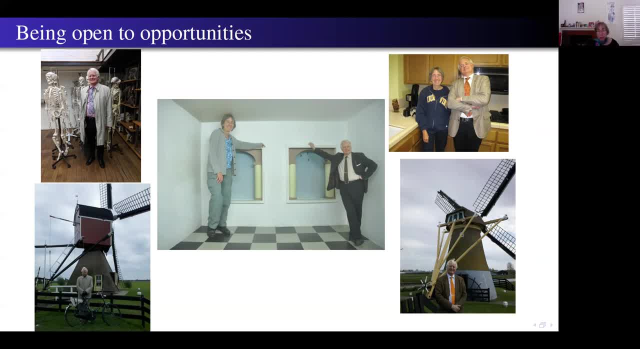 Mike Zidlow, And that led us to the cryptanalytic aspects of lattices of symmetry, which led to a long and interesting collaboration with Hendrik Leinster on lattices. So it's, you know, I kind of feel that my life has been like Alice in Wonderland: hopping. 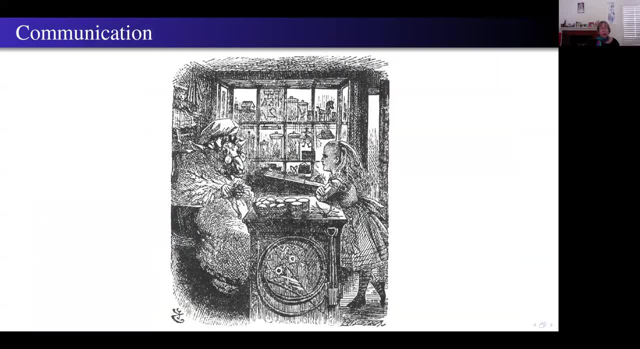 from one adventure to another. Okay, communication. So let me tell you a story. Dan Bonnet, Carl Rubin and I were working on a paper which was about composite order groups to use in pairing-based cryptography. Now, Dan wasn't being as responsive as I wanted him to be. 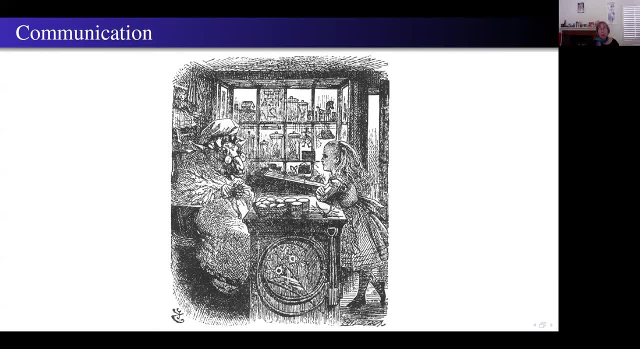 And eventually he explained to me That his highest priority is always the paper with the next deadline. So if I wanted him to work on something, I had to give him a deadline. Well, I think a few years later, Victor Miller and Neil Koblitz asked me to contribute an. 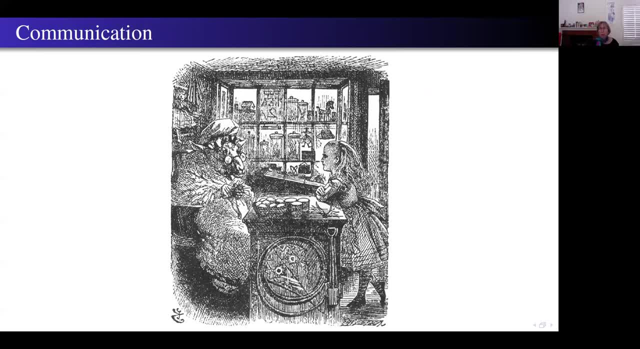 article to a special issue of the Journal of Number Theory. I think it was on the occasion of the 25th anniversary of elliptic curve cryptography. Now they said there wasn't really a precise deadline yet, maybe late spring or summer. And then later on they said: well, you know, the earliest would be, you know, the end of. 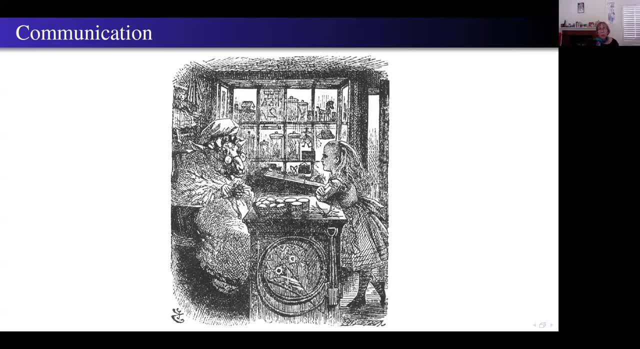 the fall. So these were not strict computer science deadlines, They were flaky mathematician deadlines. So in October I asked Neil for a firm deadline that I could tell to Dan. Neil said well, we could say the end of October, but that's clearly too soon. 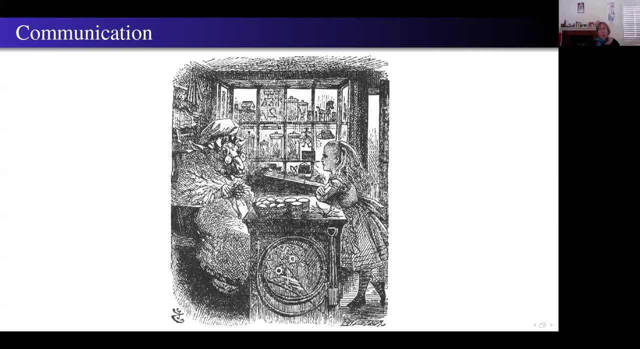 So let's say something vague, like in a few weeks. Well, I didn't think that would work on Dan, So I told Dan We have a deadline Of October 31st. Well, he worked really, really hard on that paper. 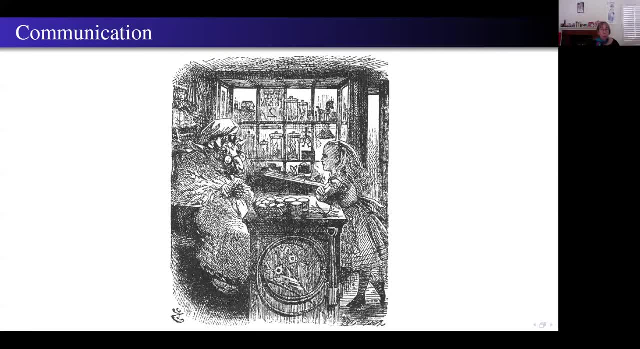 Now, on October 31st, we ran into a small obstacle, for which we needed a little bit more time if we wanted to deal with it in the right way, But Dan said: look, we have a deadline, The paper's good enough. 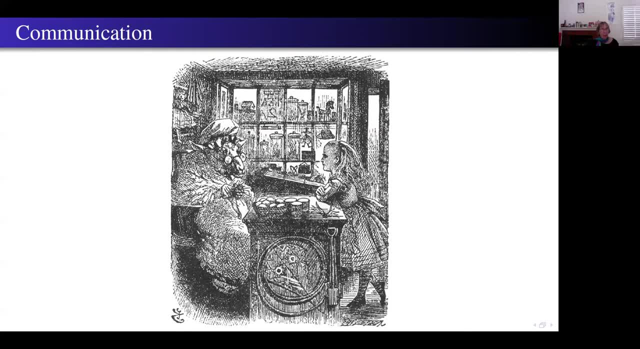 Submit, submit. Well, knowing that we didn't really have an October 31st deadline, I told Dan that I had asked the editors for an extension And they gave us an extra 24 hours. Well, in those 24 hours, we easily fixed the problem and we were able to submit a. 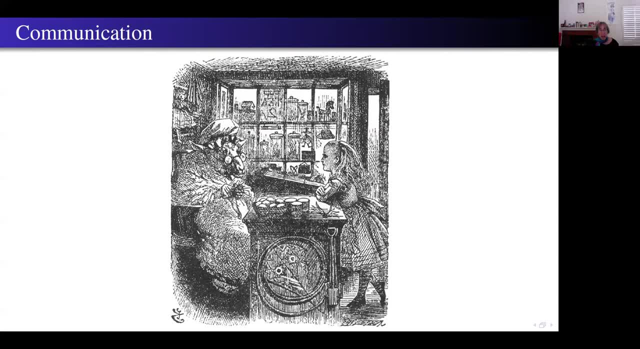 polished paper. So I must admit to this day I felt terribly guilty for misleading Dan. Now he doesn't know this story, so please don't tell him. But the point of the story is that different cultures have different ways of doing things. 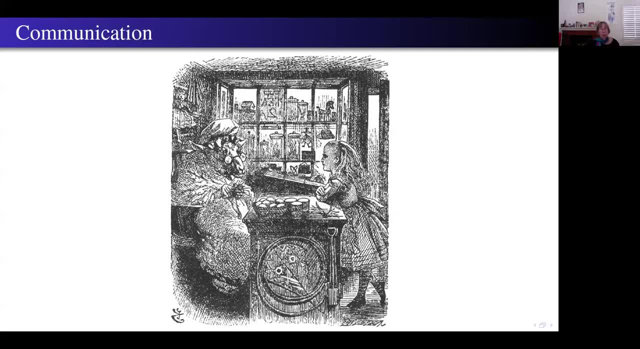 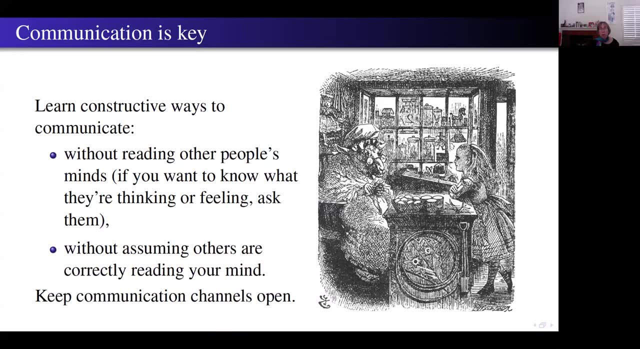 and it's important to communicate clearly and understand where the other person is coming from. So relationships are negotiations. Now, over the years, I've observed a number of disagreements in the cryptography community. Now I'm a problem solver. I like to try to solve problems. 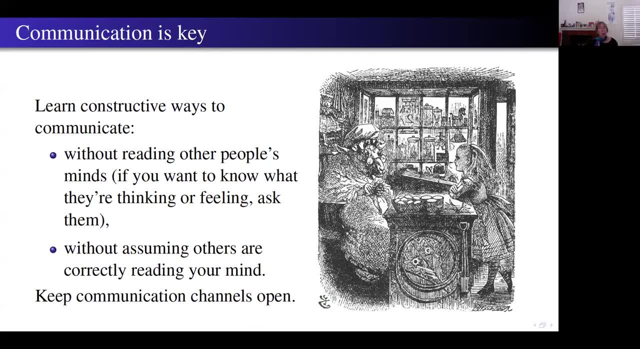 That's one reason I like doing cryptography and computer science-y things. So I tried to understand where everyone was coming from, what went wrong, what people could have done to either avoid the conflicts or make things better, And I realized that many of the conflicts came from reading other people's minds and 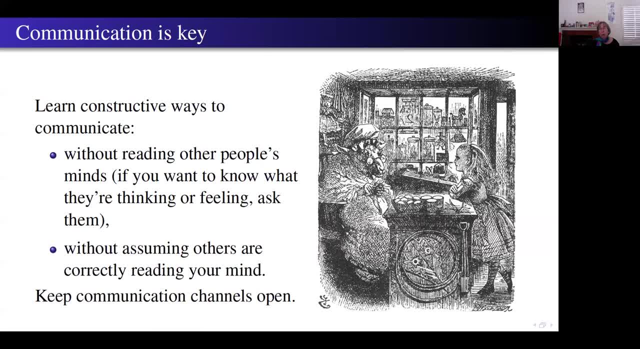 describing bad motives to them and from assuming that others could read your mind and know what you're thinking and why you're angry with them. So when I was first asked to review a cryptography paper for a conference proceeding, I refereed it the way I would a math paper. And when I sent my 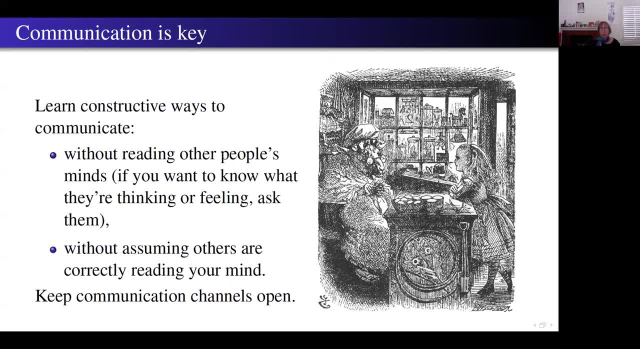 report. to the person who had asked me to review the paper, he said: oh, that deadline already passed a long time ago. Your review is too late to be helpful. So at that time I didn't realize that in his field reviews need to be quick and there are deadlines for the reviews And it never. 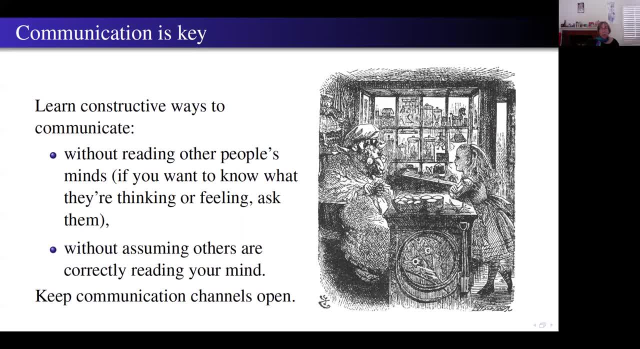 occurred to him that I didn't know that and that he should tell me what the deadline was. So he thought: you know, everybody knew that. Everyone knew what conferences was and knew when the deadline was. So clear communication is important, especially with people in a different 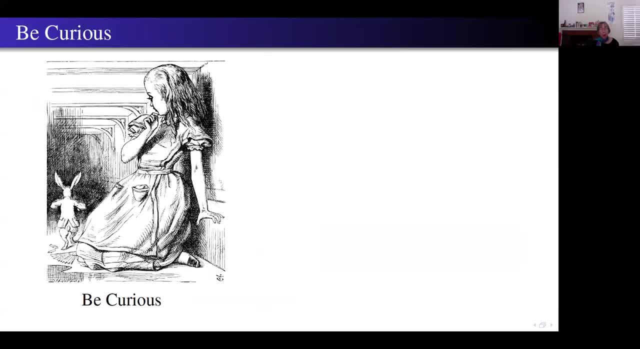 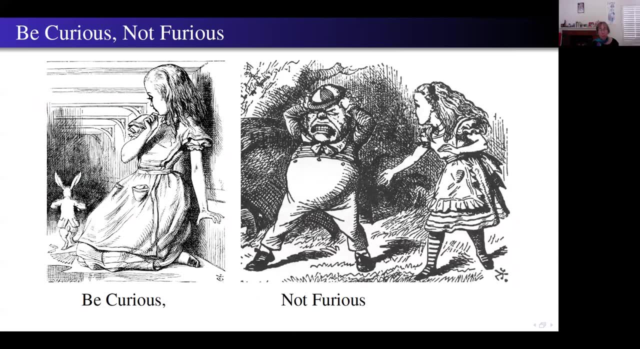 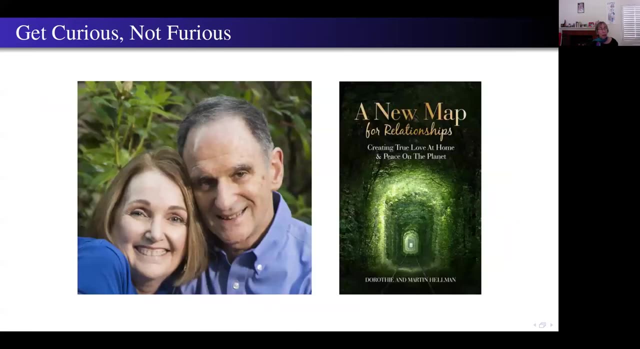 field or a different culture. So I've talked about being curious and open to opportunities. In particular, be curious and not furious, And here I should credit Dorothy Hellman and Martin Hellman. Their wording was actually get curious, not furious, And I highly recommend their book A New Map for Relationships- Creating True Love at Home and 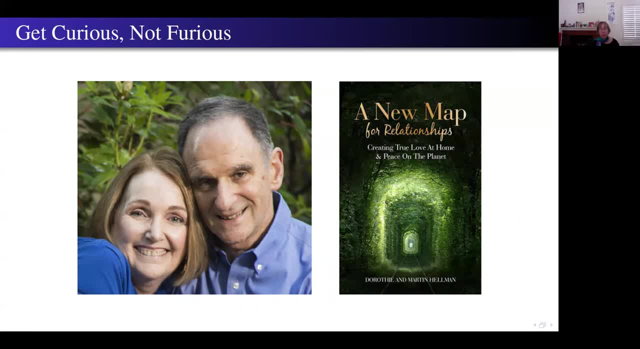 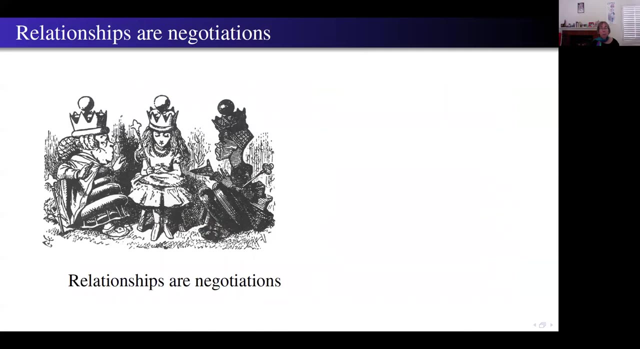 Peace on the Planet, in which they say that by getting curious and not furious, you can not only improve your personal relationships and your work relationships, but you can also have peace on earth. So I believe you can still download this free online. So relationships and negotiation is not ultimatums. as I said, It's a useful 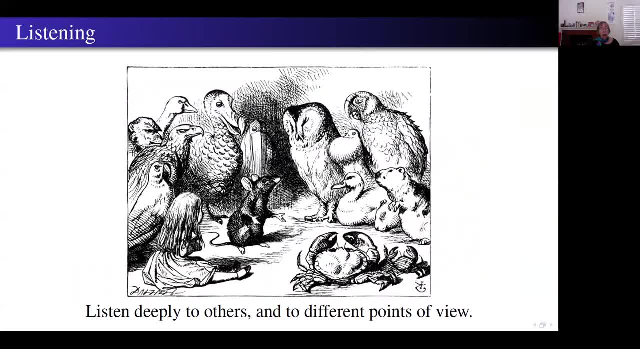 thing to keep in mind. Now I would like to emphasize the importance of listening, And I can't really emphasize this enough. I think the world would be a lot better if people talked less and listened more. So you learn a lot more by listening than by talking. 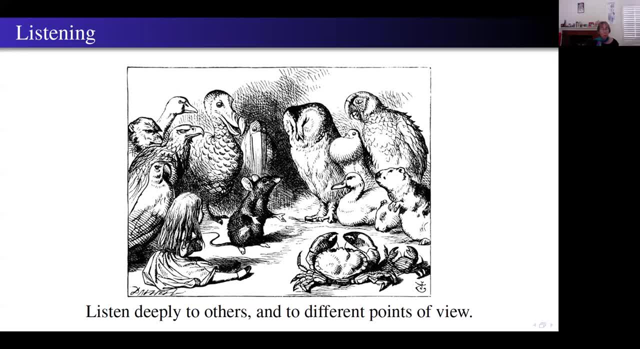 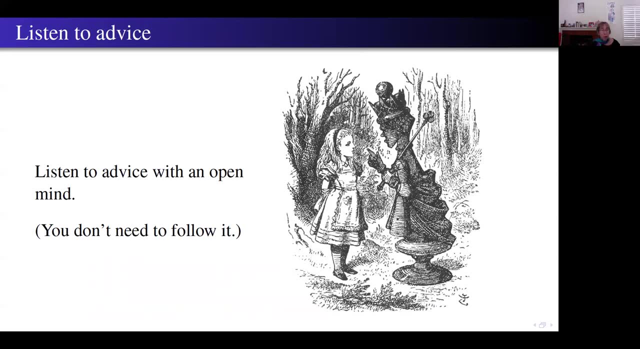 So a lot of us have been on committees. We kind of wish that people would talk less, listen more and learn from the other people around them. So, in particular, listen to advice with an open mind. You don't necessarily have to follow. 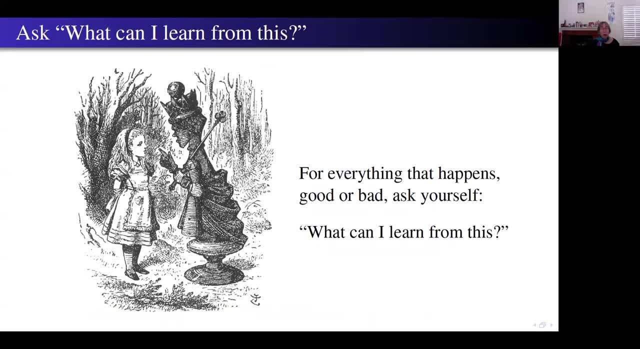 it. But you can ask yourself: what can I learn from this? So, for everything that happens, good or bad, I find it constructive to ask myself: what can I learn from this? Everything I read on the internet, rather than getting furious, I'm going to ask myself: what can I learn from this? 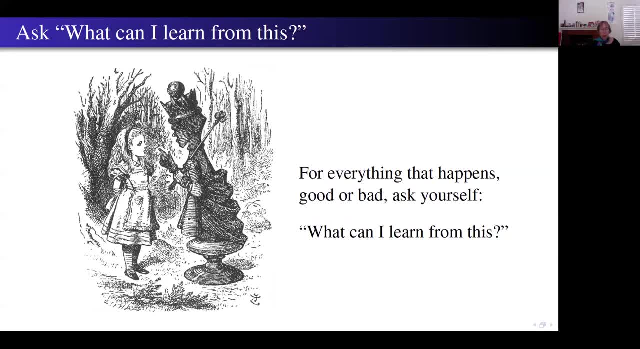 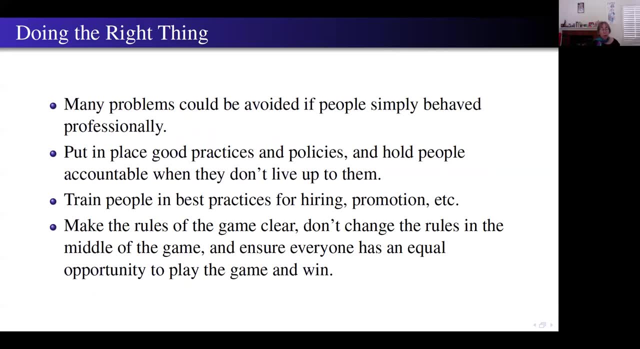 Getting angry with it, I think, but is there something useful I can take away from it? So sometimes people ask me for advice. Sometimes they give advice I'm not asked for and I'm trying to learn not to do that. But when you're invited for an hour talk, I figure, okay, I can give you. 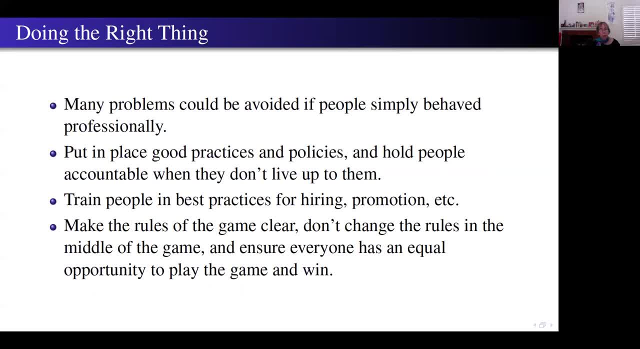 some advice. So the advice I give when people ask me for it is well, many problems could be avoided if people simply behave professionally. So we like to think of our colleagues as being our friends, But it's important to remember that we have a professional relationship with our coworkers and we have an 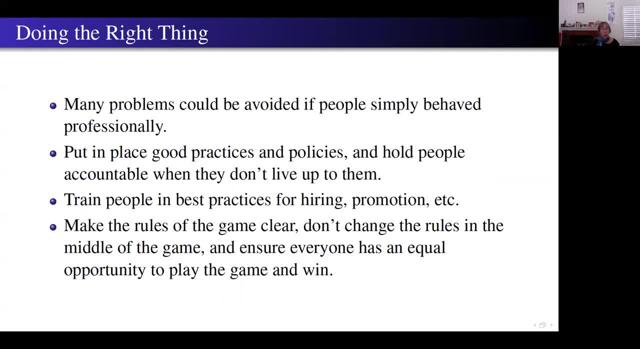 obligation to behave professionally, So sometimes it's useful to think: am I behaving professionally? Is this a professional way to behave? Put in place good practices and policies. Hold people accountable. Train people in best practices, So this includes for hiring and promotion, for teaching. 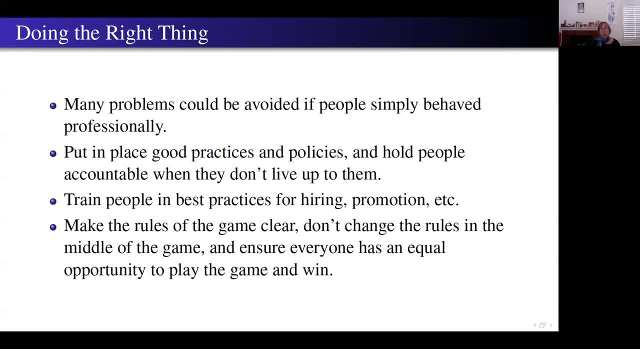 for choosing students, for choosing interns, And something that I find very important is make the rules of the game clear- Don't change the rules in the middle of the game- and ensure that everyone has an equal opportunity to play the game and win. So an example of this is in hiring, where the public criteria given in the job ad 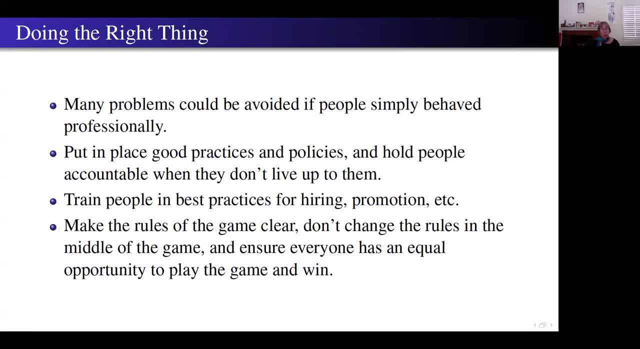 can sometimes be quite different from the secret criteria or the real criteria for the job, And the people in the right circles know the real criteria and have an advantage. So I've actually seen this a lot And if you want more stories about this, 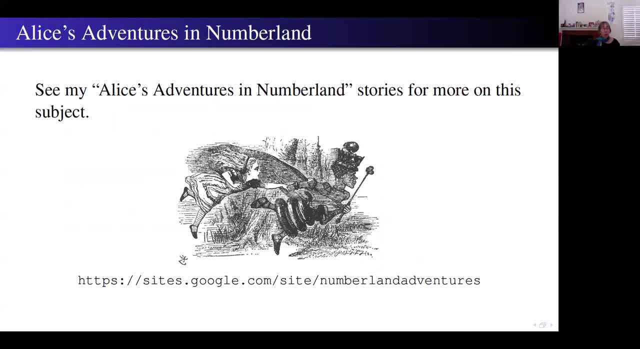 I would send you to my Alice's Adventures in Numberland website in which I tell some more stories. So in general, what I advise people is to keep in mind that people need to see problems getting fixed so that they can trust that if they. 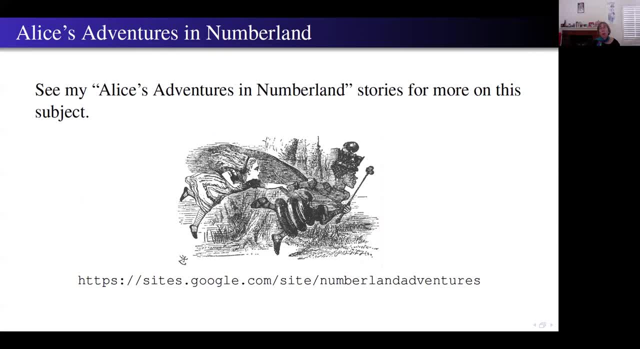 bring these problems to the attention of people in authority, that things will get better rather than getting worse. And also senior people need to step in when there's a problem. So when the leaders of the field in the field don't step in to do the right thing, everyone sees that and it can be demoralizing, especially for the junior people. So I'm 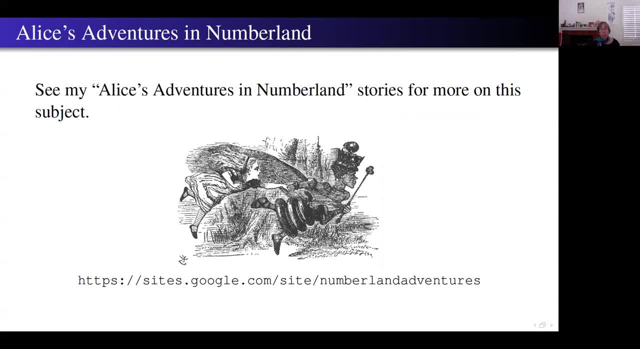 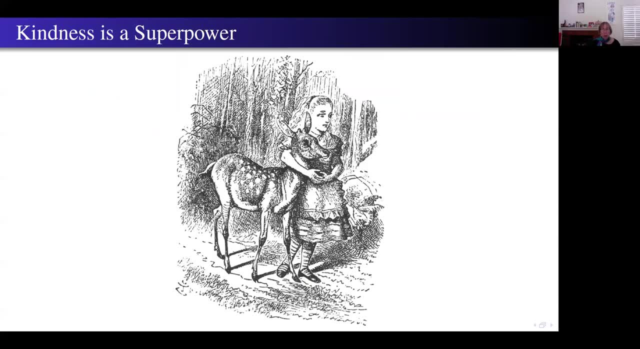 glad that various communities, including the IACR, are thinking about a number of these issues. Given the stress that everyone is under now, it's especially important to be kind. So a friend and colleague of mine, Shahed Sharif, pointed out to me that kindness is a superpower. I was on a campus-wide committee that ran a committee of